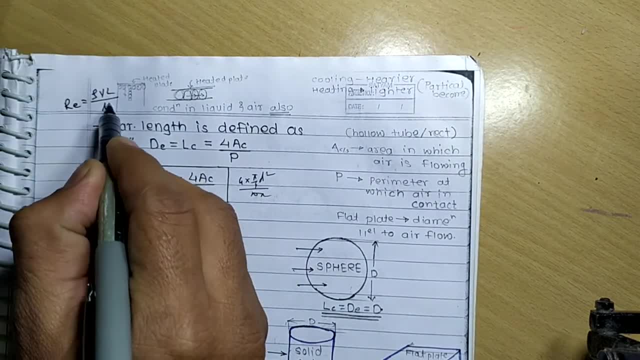 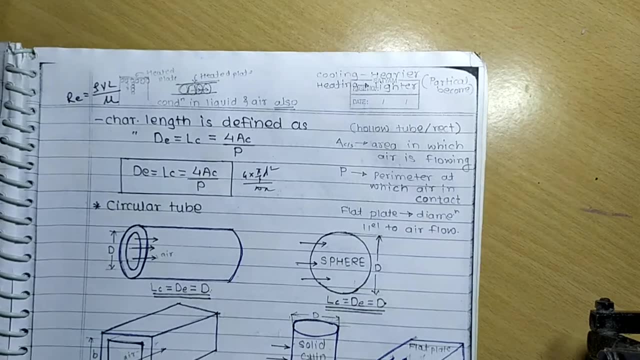 Re is equal to rho VL by mu. That is the formula we are knowing. In this L, we have written What is L. L is the characteristic length. L is called as characteristic length. Now, what is characteristic length? That we have to understand Because when solving a problem, 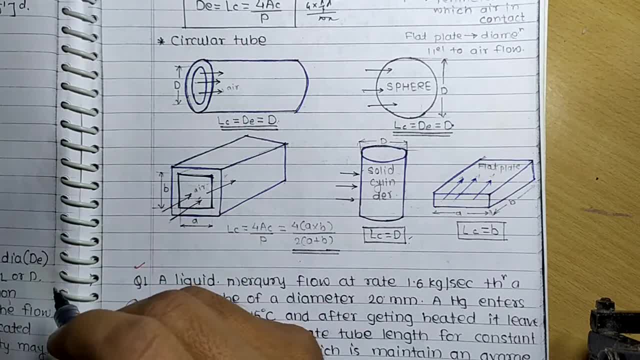 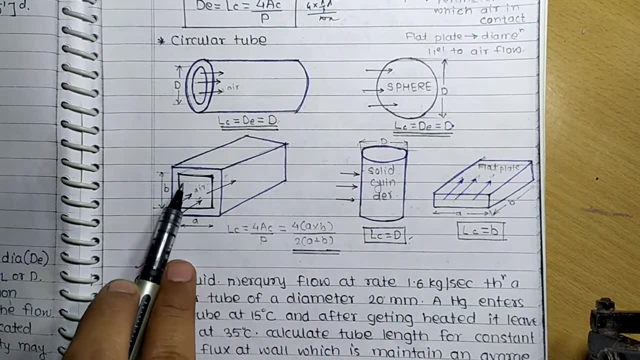 we are using a formula, and in the formula I should put value of L. So there are some standard geometries, as I have shown you. That is, circular, tube sphere, solid cylinder, flat plate and square or rectangular duct. These are some. 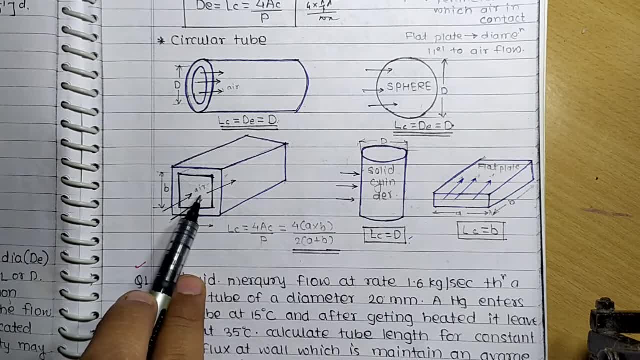 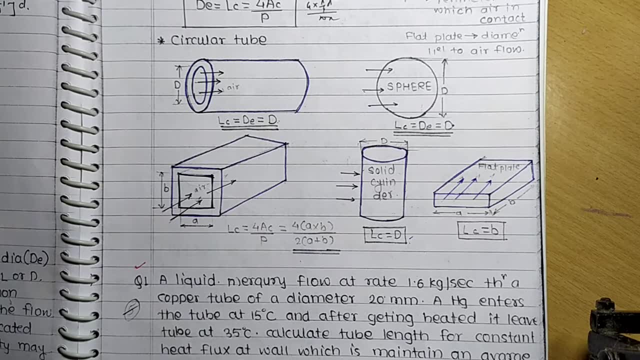 standard geometries in which we have to identify what is characteristic length. Basically, characteristic length can be denoted by capital: L or LC or DE. LC indicates characteristic length, DE indicates equivalent diameter. So here you can see: LC is a characteristic length. So here you can see LC is a characteristic length. So here you can see LC is a characteristic 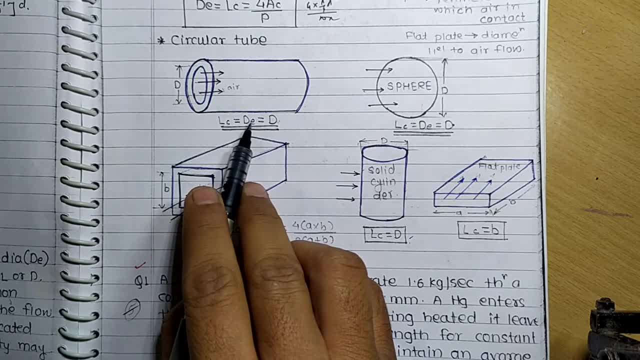 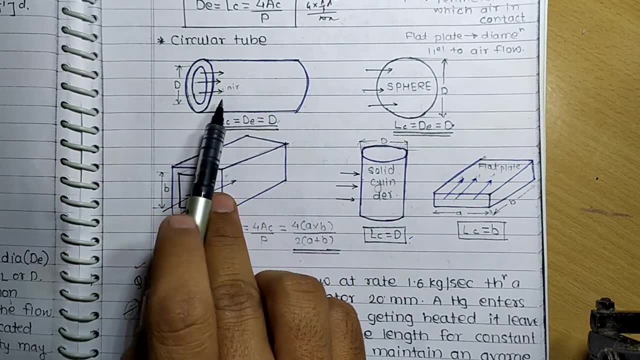 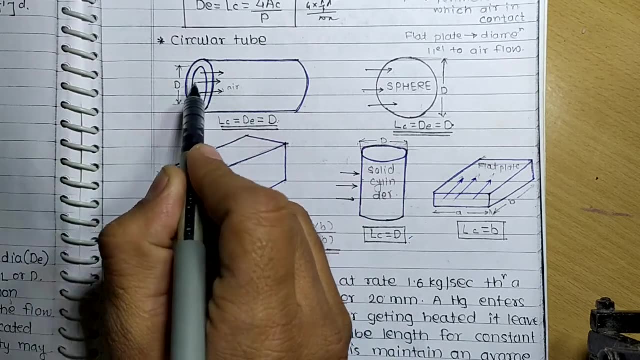 length, or DE is also called as equivalent diameter, but both are same. When you are having a circular tube like this, when you are having a circular tube like this in a circular tube, if the air is flowing like this, which may be driven by a blower, etc. So when air is, 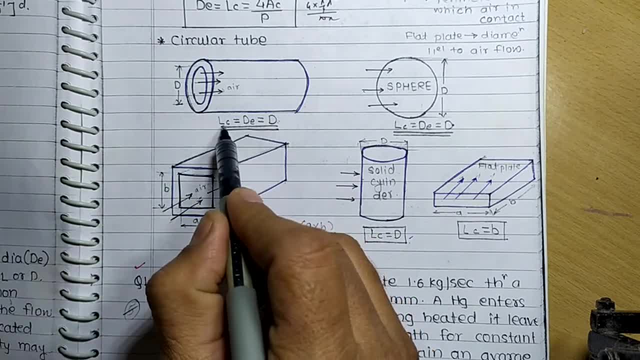 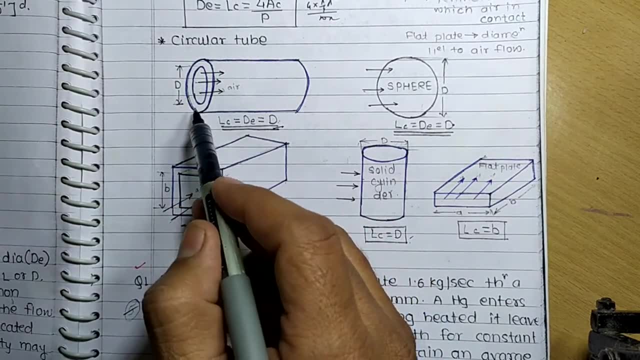 flowing through this one, then the characteristic length is a diameter of tube. Here we have written: LC is equal to DE is equal to D. So whenever there is circular tube, we should take inner diameter as a characteristic length. Whenever there is a sphere, once again characteristic length or equivalent diameter is nothing but. 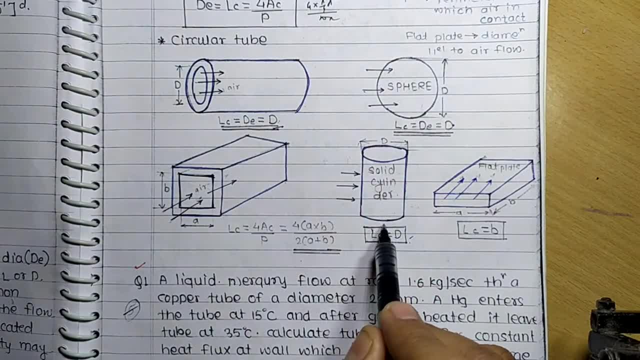 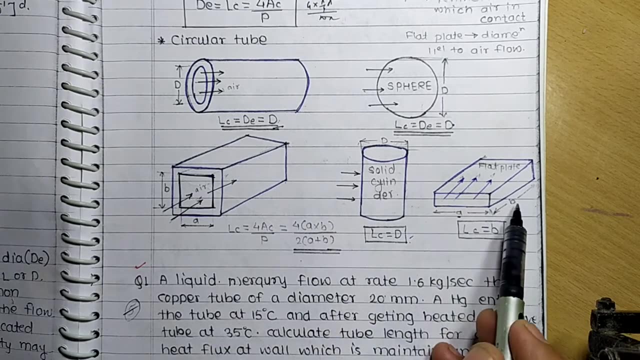 a diameter of sphere. When we are having a solid cylinder kept on a base and air is flowing across, that at that time also, characteristic length is nothing but a diameter. When we are having a flat plate in the flat plate, let's consider, this is dimension A, this is 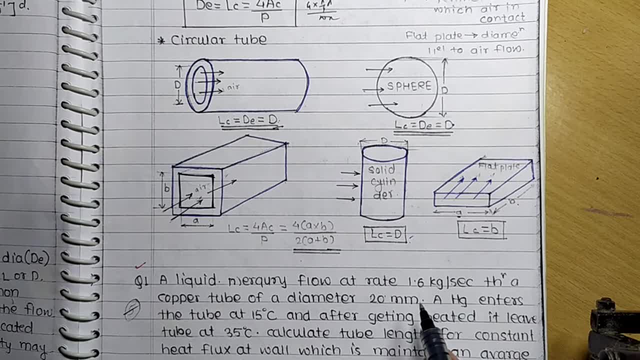 dimension B, Then the dimension which is parallel to air flow direction is called as characteristic length. Now I have shown you. air flow direction is like this. Now to the air flow direction, the dimension which is parallel to this one is B. So this is B, So 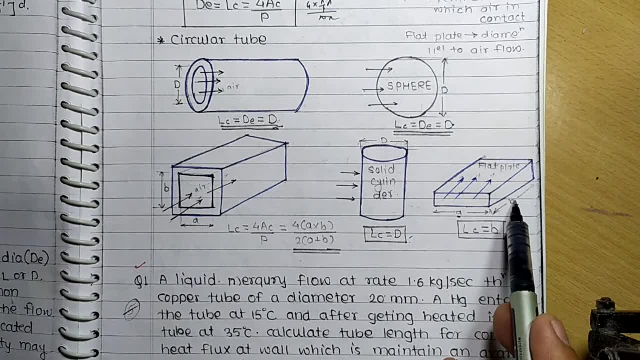 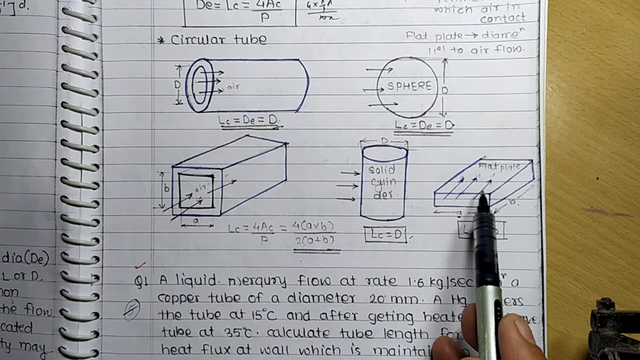 in the current case the characteristic length is B because air is flowing parallel to B. Now if I take the air flow in this direction like horizontal, so when it is flowing horizontally, then the characteristic length will become A. So you have to remember, for flat plate. 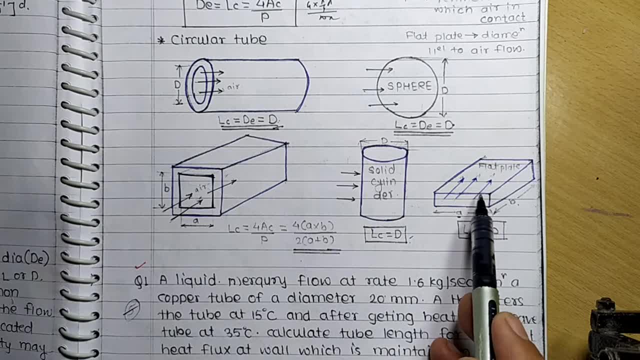 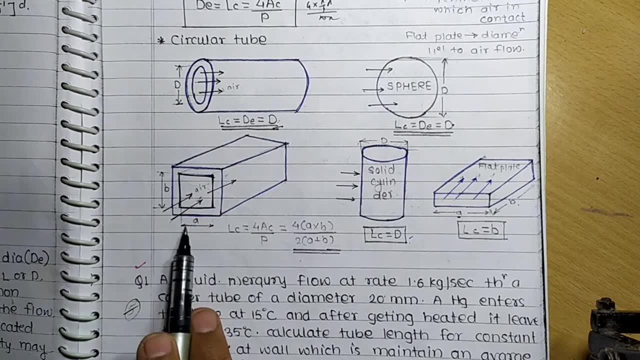 the dimension which is parallel to air flow direction is called as characteristic length. When we are coming square or rectangular duct which has dimension A and B, A is inner dimension and B is also inner dimension. At that time the characteristic length will become 4AC. 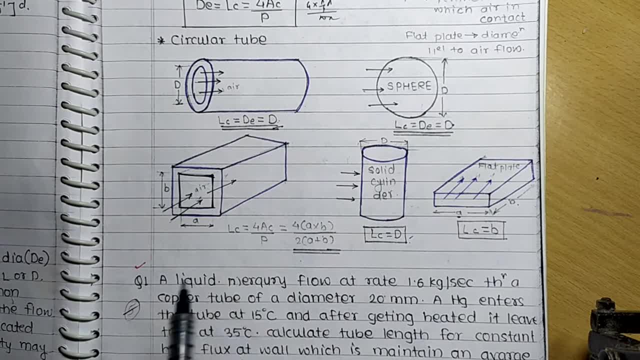 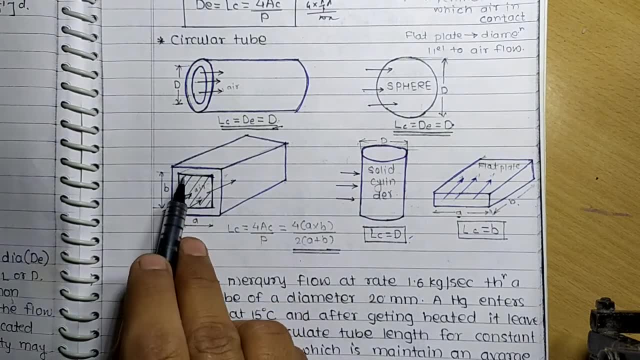 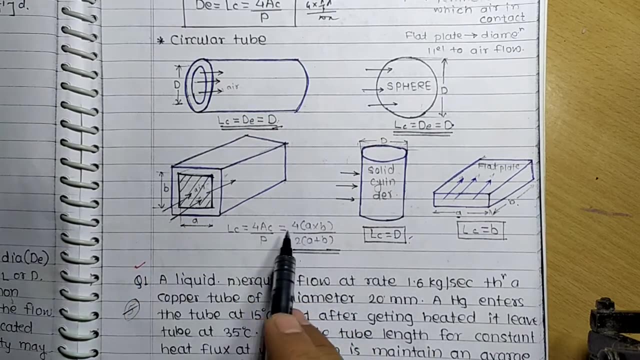 by P. What is AC? AC is cross sectional area, So cross sectional area is this one. This is cross sectional area. So 4AC by P perimeter is nothing but summation of all these four sides. So here we have written that, if there is, this is rectangular duct, cross sectional. 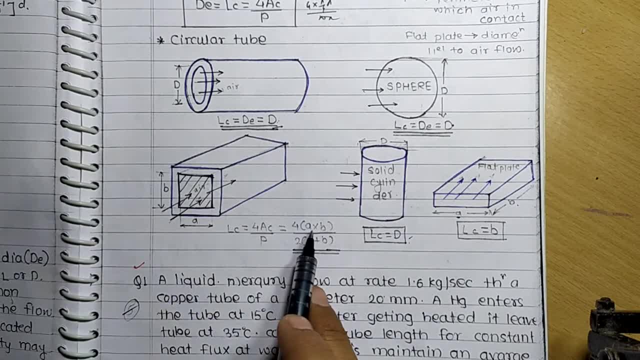 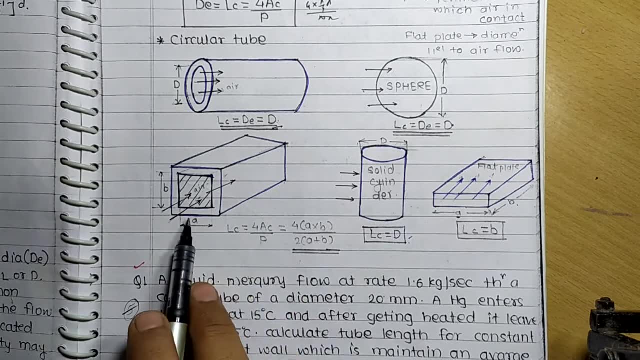 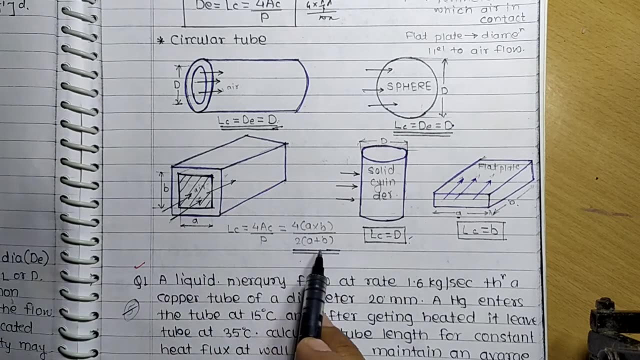 area will become A into B. Cross sectional area will become A into B. So rather than AC I have put A into B. Perimeter will be what Summation of four sides? So that will become A plus B, plus A plus B. or I can write 2 in bracket, A plus B, Right? So these are. 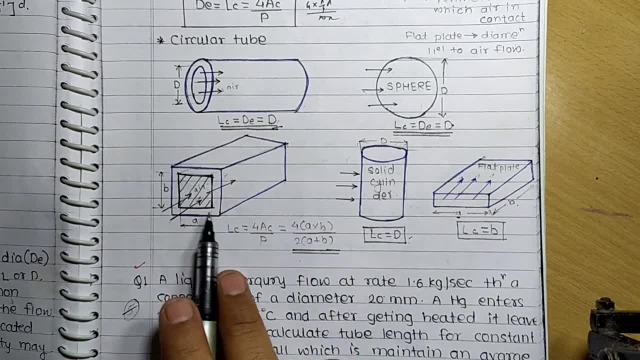 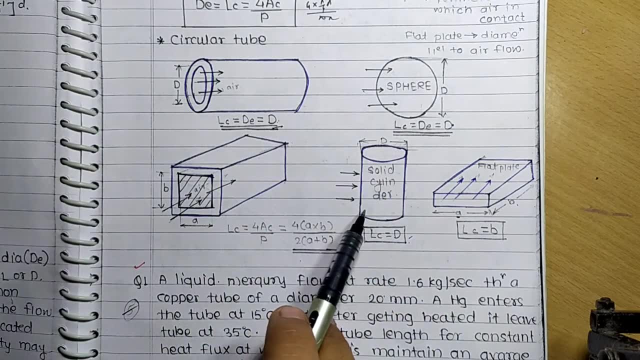 what Various characteristic length. In case of duct, that is 4AC AC by P, Whereas other it may be circular tube, it may be sphere, it may be cylinder kept or base. It's a diameter. In case of flat plate, it is a dimension which is parallel. 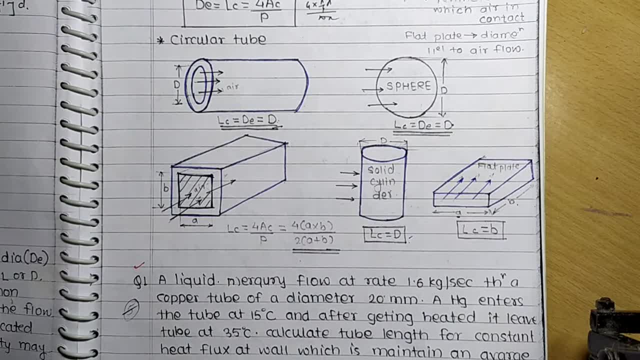 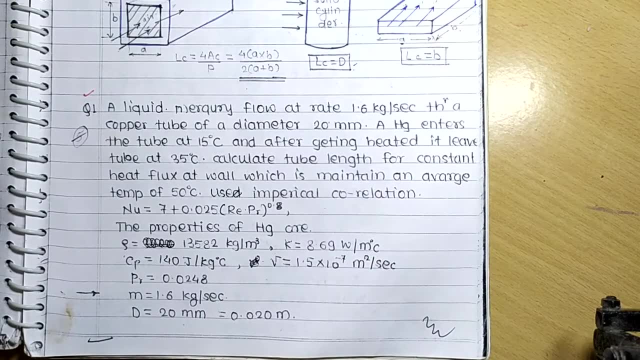 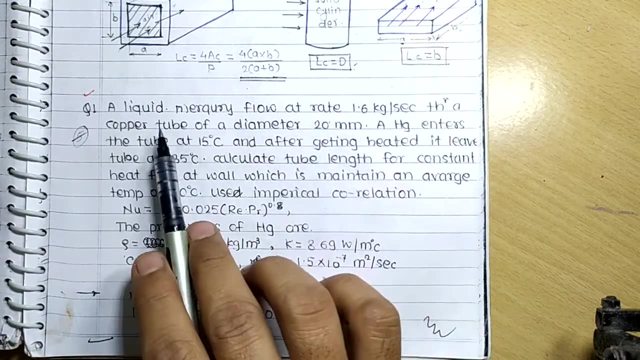 to air flow direction. Okay, So this knowledge will be very useful for solving problem of force convection. Now let's go for solving a problem. Let's see the first problem. what they have given? A liquid mercury flow at rate of 1.6 kg per second through a copper. 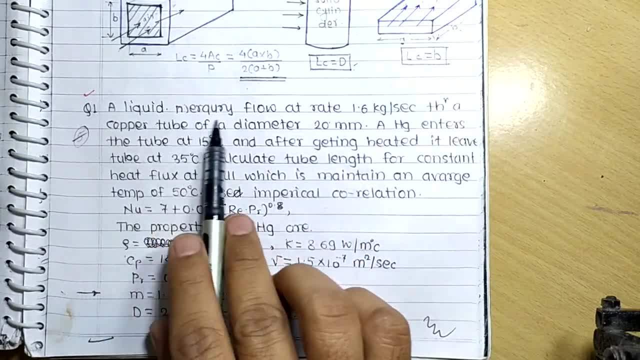 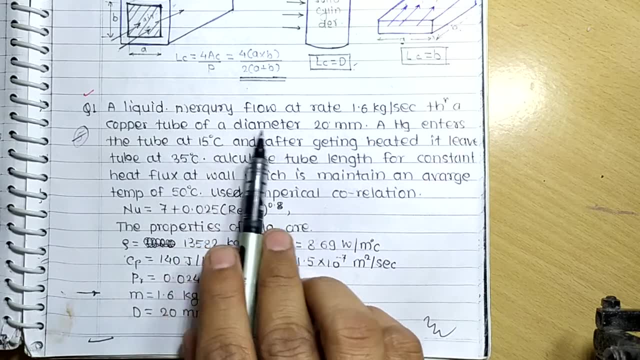 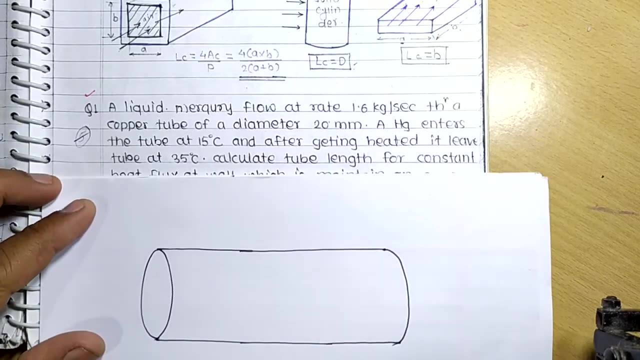 tube of diameter. So fluid which we are considering is liquid mercury, whose flow rate is given 1.6 kg per second through a copper tube of diameter 20 mm. Let's consider this particular pipeline now. So I will run the pipeline as like this. So let's consider this is the pipeline through. 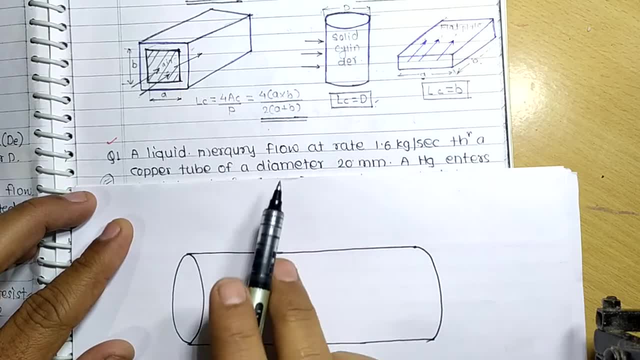 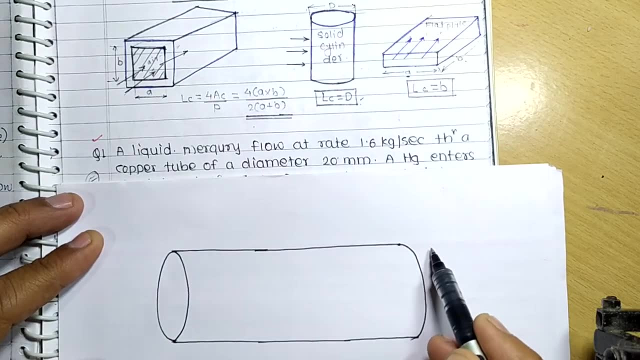 which mercury is flowing Through which mercury is flowing Right. So liquid mercury flow at rate of 1.6 kg per second through a copper tube diameter 20 mm. Let's consider the inner diameter Near the inner diameter of this copper tube is how much Is the 20 mm? We know that all. 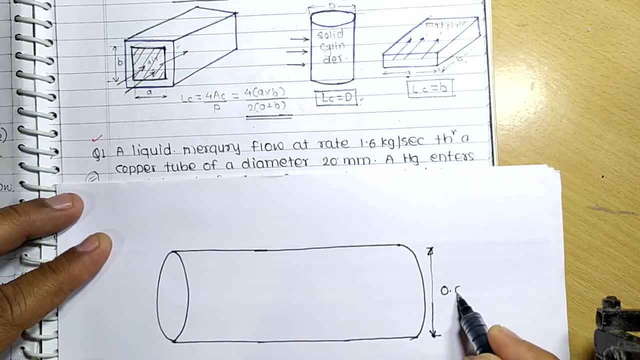 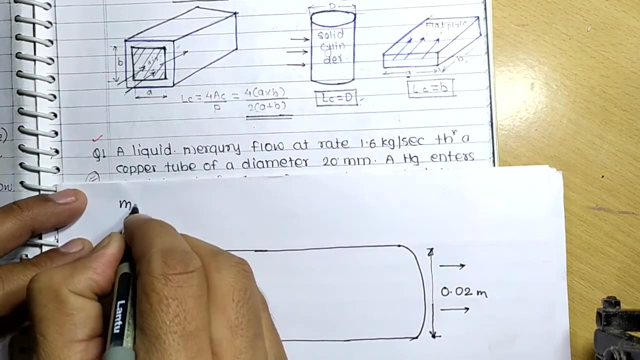 dimension we take in meter, So I'll write here 0.02 meter. So what I've done? I have converted 20 mm into meter And through that mercury is flowing. So mercury enters at this point and it leaves at this point. Right Now, mass flow rate of this mercury is how 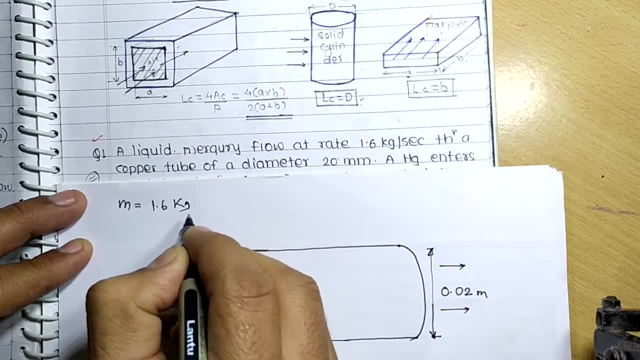 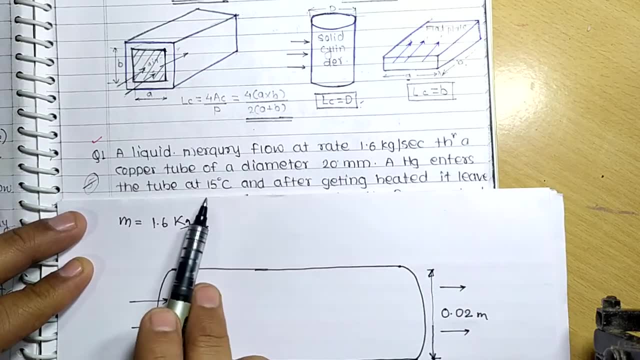 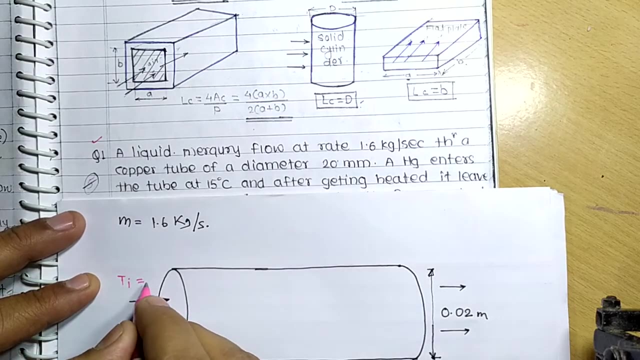 much. Mass flow rate is 1.6 kg per second. Okay, second, okay, that's the mass flow, right? okay? a hg enters tube at 15 degree celsius, so entry temperature of hg. so let's consider ti, ti, which is equal to 15 degree celsius in the temperature. 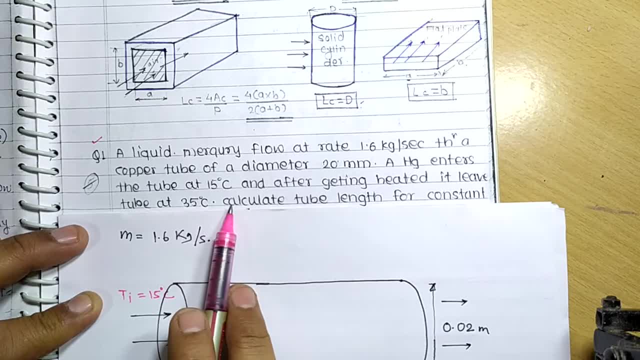 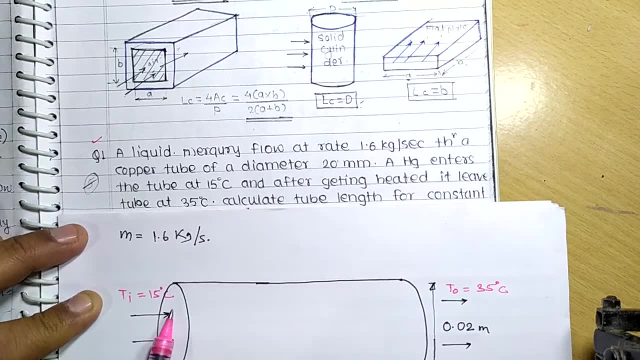 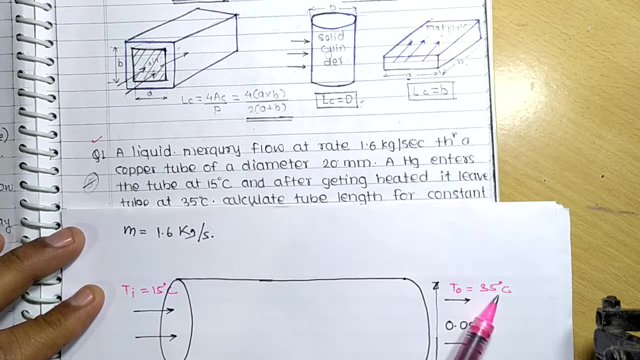 and after getting heated it leaves the tube at 35 degree celsius. so at the outlet, what we are getting? temperature which is 35 degree celsius. so when mercury enters at 15 degree celsius, it will get heated and after getting heated it will be left by temperature of 35 degree celsius. 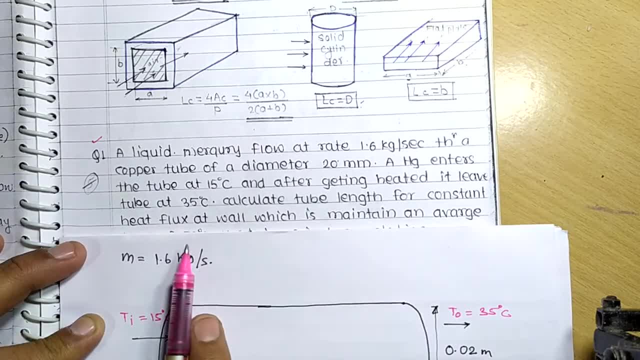 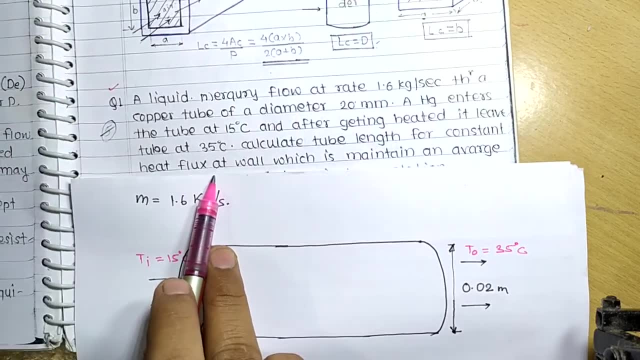 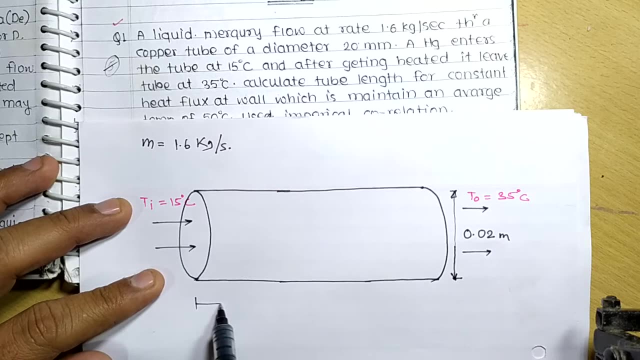 okay, calculate tube length for constant heat flux at wall which is maintained at average temperature of 50 degree celsius. so what we have to do, we have to determine a length of pipe. we have to determine what length of pipe, so it will have a length as like this: so let's consider: 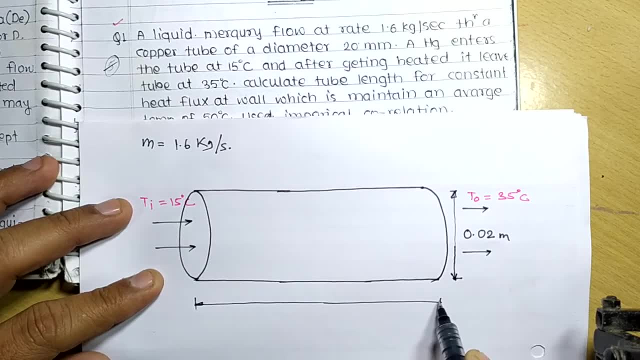 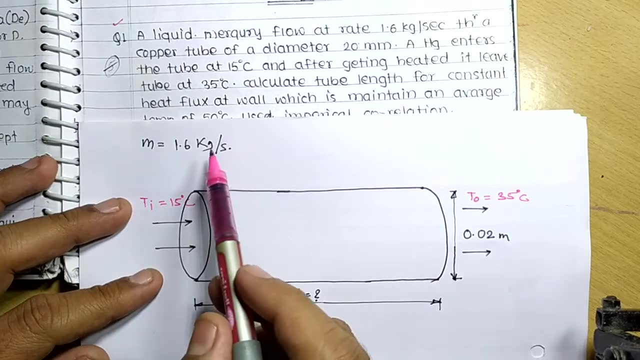 this is the complete length of tube. okay, we have to determine this length. we have to determine this length when the tube temperature, tube temperature is given to you 50 degrees celsius. here it is given 50 degrees celsius, so i'll write: 50 degrees celsius is. 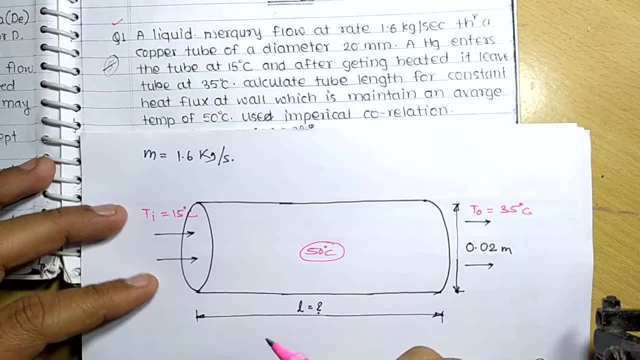 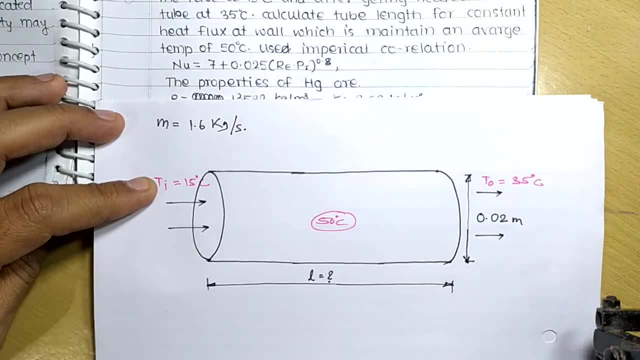 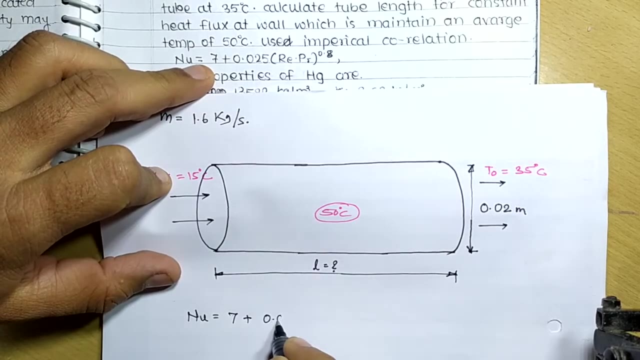 tube wall temperature. okay, next, what they have given, use empirical correlation. so they have given one empirical correlation. that correlation we have to use it. so i'll write here: empirical correlation: nusselt number is equal to 7 plus 0.025 re into pr raised to 0.8. that's the correlation. 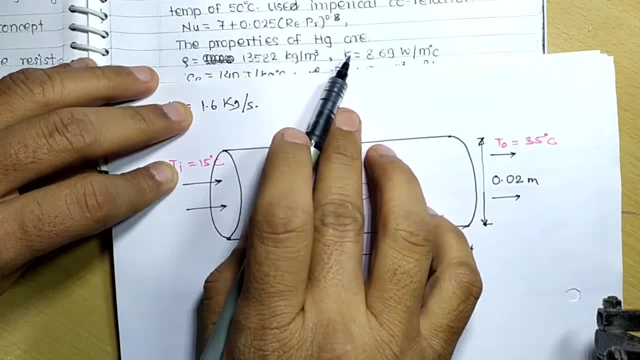 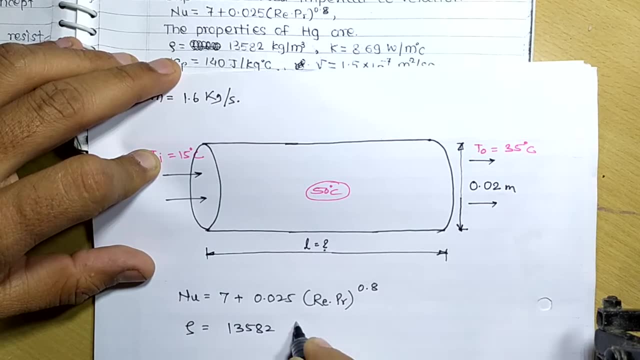 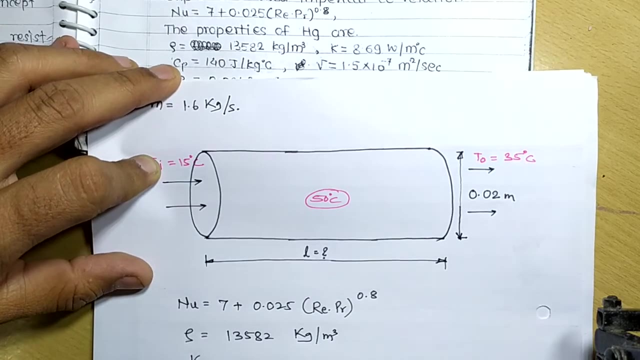 given to you the property of hgr. they have given the property of hg, that is mercury, that rho is equal to 1, 3, 5, 8, 2 kg per meter cube. that's one property given. next, thermal conductivity k is given. what is thermal conductivity k? in this case the k. 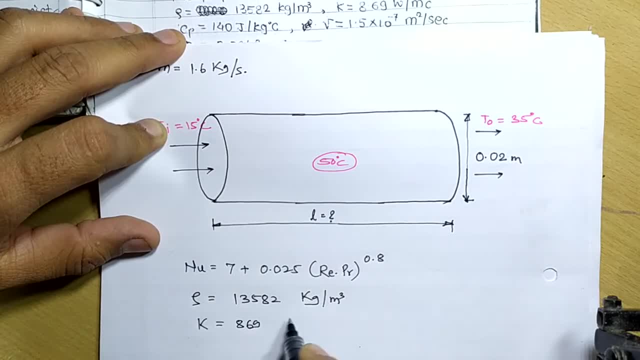 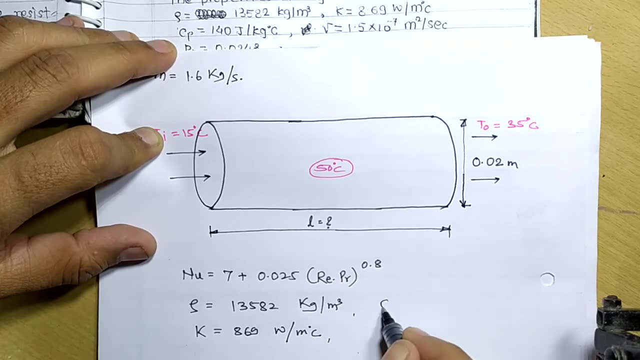 is equal to 1, 3, 5, 8, 2 kg per meter cube. that's one property given. next, thermal conductivity k is nothing but 869 watt per meter per degree celsius. that is the thermal conductivity given. next cp is given. so what is cp? cp is 140 joule per kg per degree celsius. then nu is given, that's. 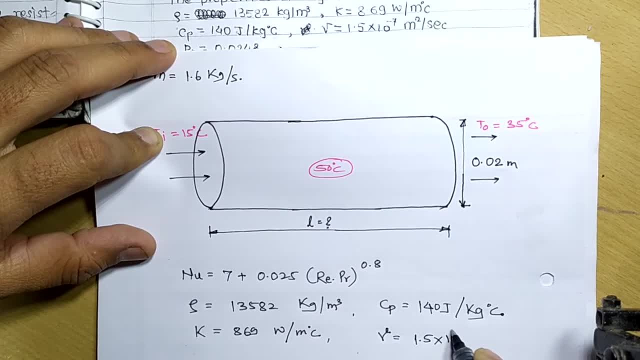 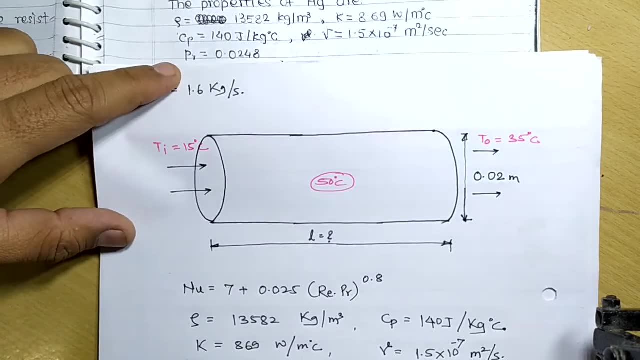 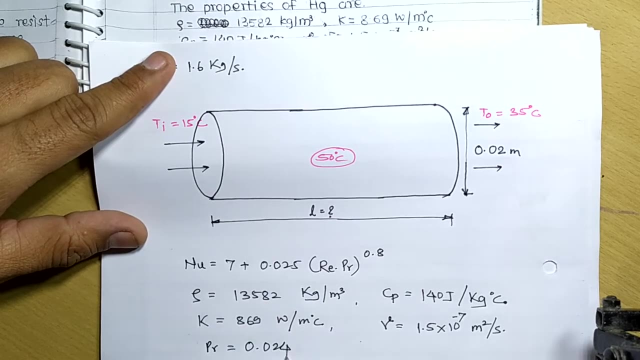 nu and nu is nothing but 1.5 into 10, raised to minus 7 meter square per second. okay, and the frontal number is also given. this is the parental number. so parental number is given to you. parental number is given to you. how much, 0.0248, so this, all these properties of mercury, is given to you. so by 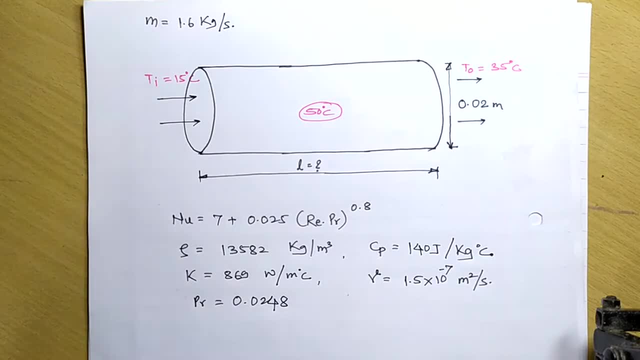 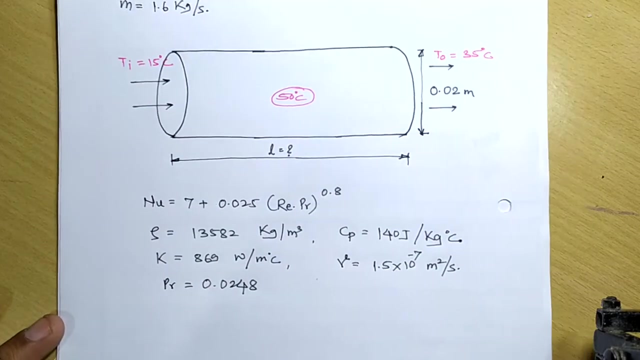 using all this given data. by using all this given data, what we have to do? we have to solve a problem for determination of length of pipe, for determination of what length of pipe? let's go for solving this. let's go for solving this now. we can solve this particular problem by using the equation that's what called as cooling law. 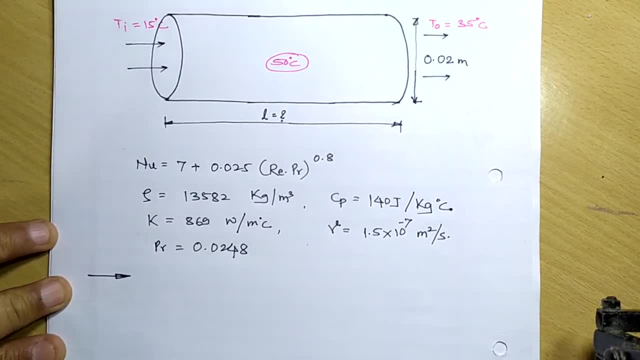 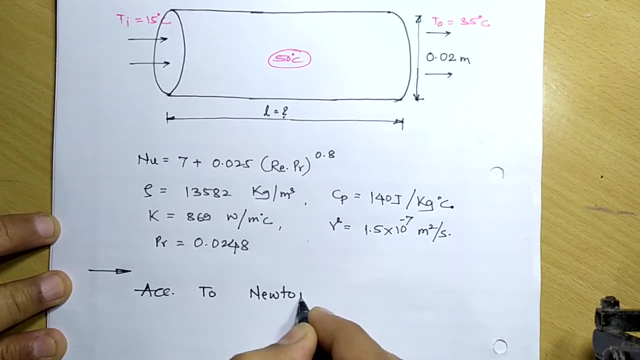 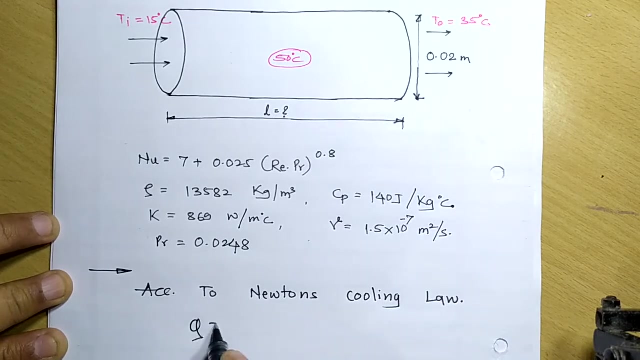 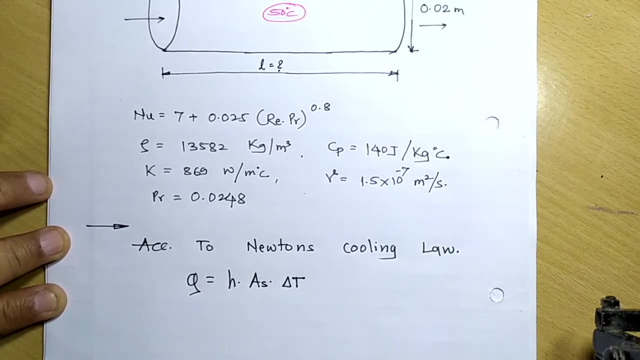 newton's cooling law. so let's go for a solution in the solution we'll go for according to newton's cooling law. according to newton's cooling law, what says newton cooling law? newton cooling law says q is equal to q is equal to h. a, s, delta, t. what is a, s, a s is surface area. so we can solve this. 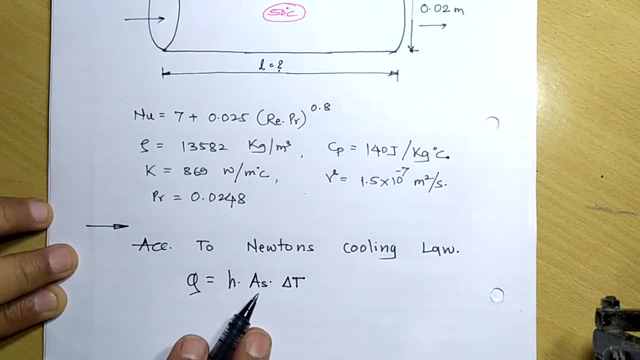 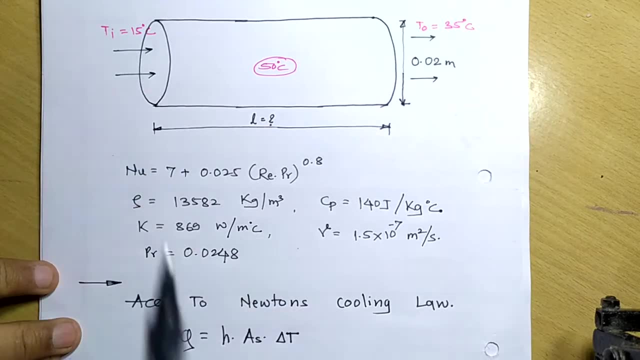 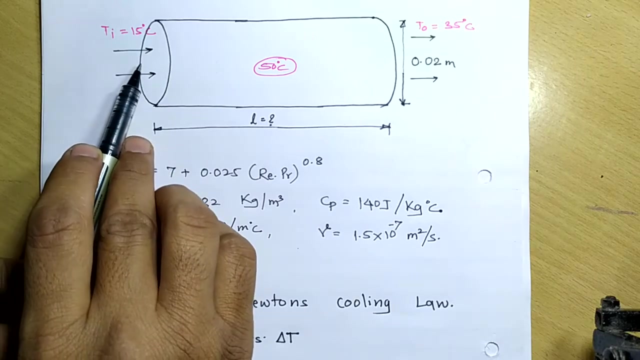 here. yes, q is heat transfer, h is heat transfer coefficient, a, s is surface area and delta, t is temperature difference between hot body and cold body. now, if you check out the given data, what is the surface area to which mercury is coming in contact with the pipe? because in this 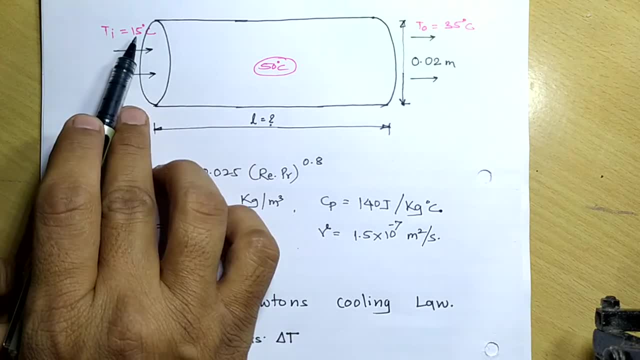 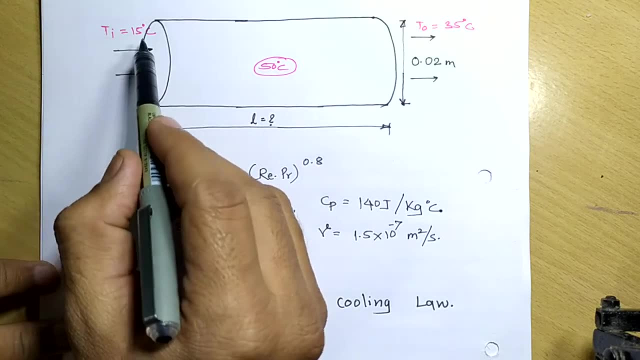 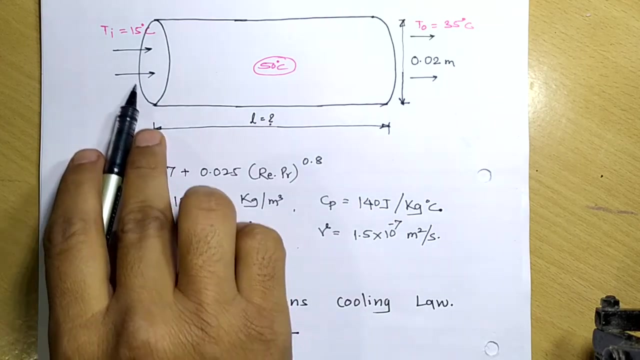 case, the pipe hits the mercury. pipe hits the mercury, so what is the area of pipe which is coming in a contact with mercury that we have to find out? if you observe very carefully, the inner fragment of this particular pipeline is called as, so the inner surface area is contact with the. 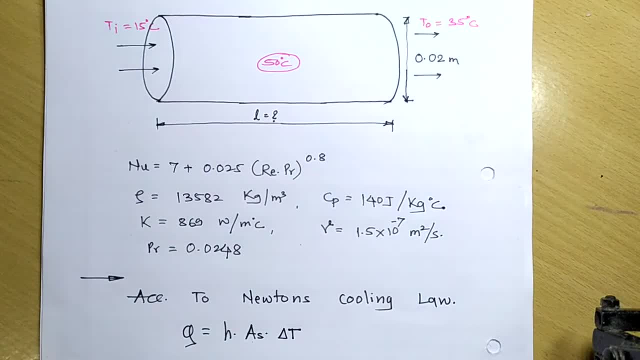 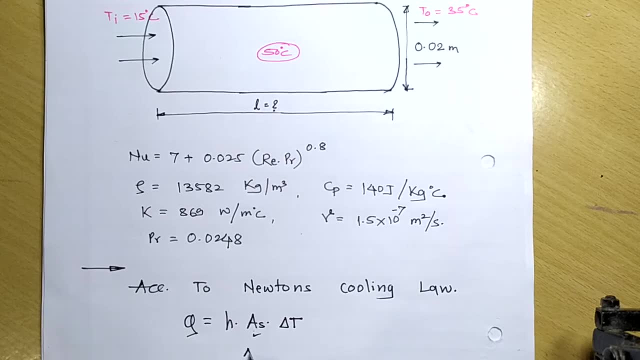 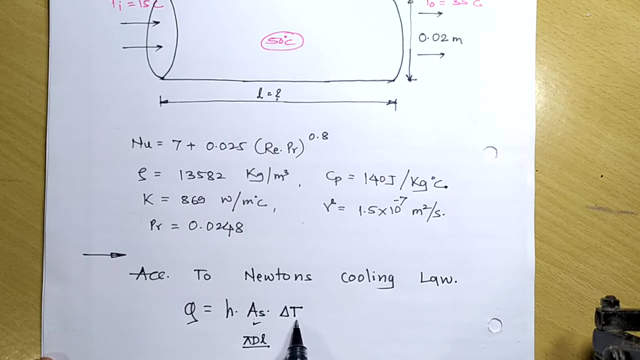 mercury. what is in a surface area perimetral length that we are. so this surface area is perimetral length. so perimetral is pi d and length is l. so the surface area, I can write pi d, l. that's the surface area. what is the temperature difference? temperature difference is nothing but. 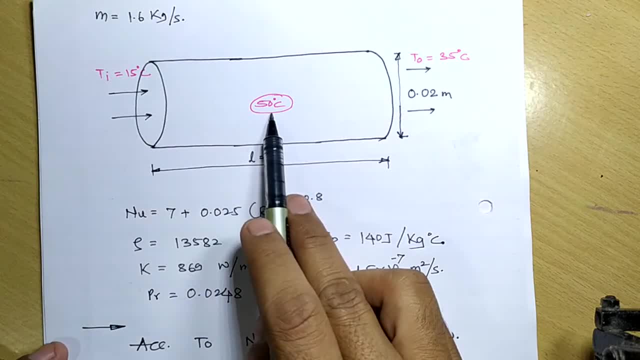 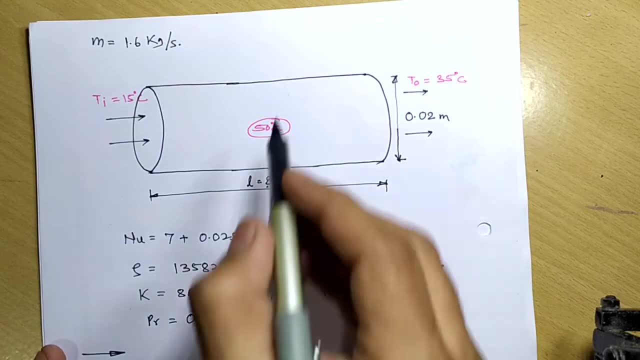 temperature difference between hot body and cold body. what is the body? hot body is the, the liquid pipe. cold body is the mercury, but mercury temperature is not constant. mercury temperature is not constant. i can write here that hot body temperature is 50 minus. what is cold body? 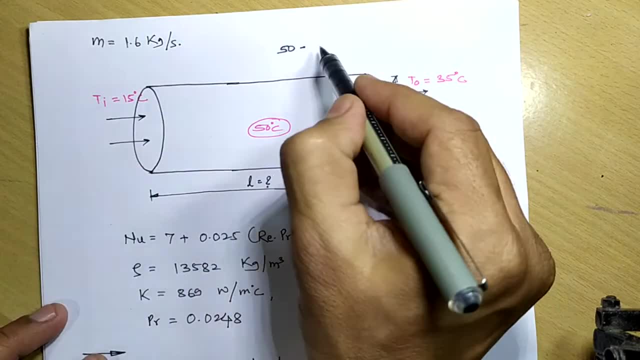 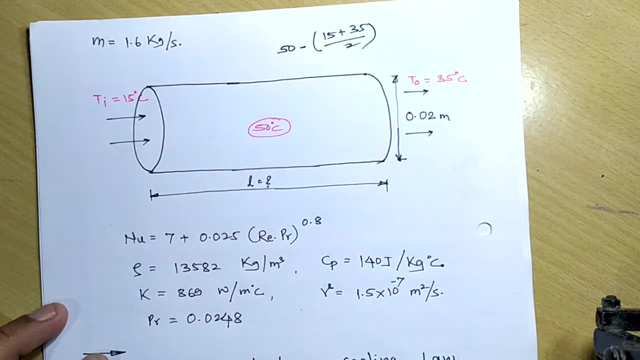 temperature- cold body temperature- is varying continuously and that's why i am going to take it average. so what will be average? 15 plus 35 by 2? that is also called as bulk mean temperature. that is also called as bulk mean temperature. okay, so delta t is known now. delta t is known now that. 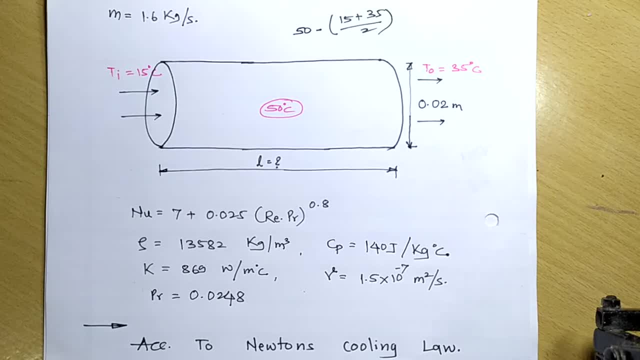 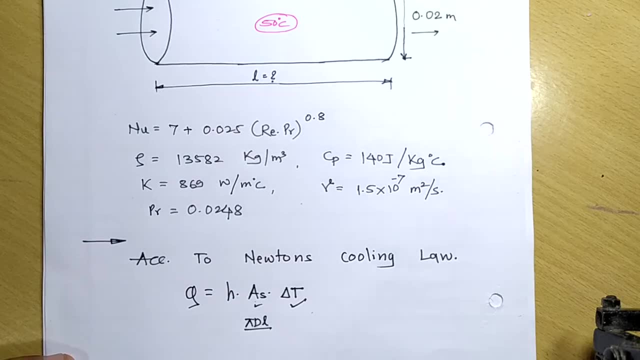 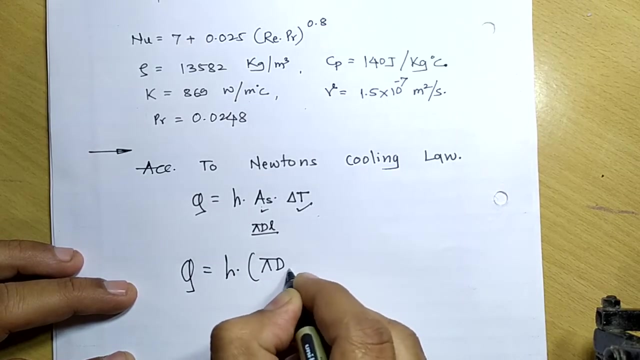 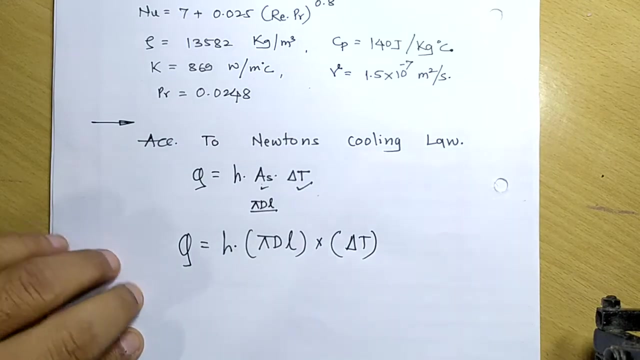 50 minus 15 plus 35 by 2, h is heat transfer coefficient, q is what heat transfer, q is what heat transfer. now, in the current problem, this formula i can write, modify or updated as h, pi, dl into delta t. now in this, in this i am knowing, the value of pi is constant. 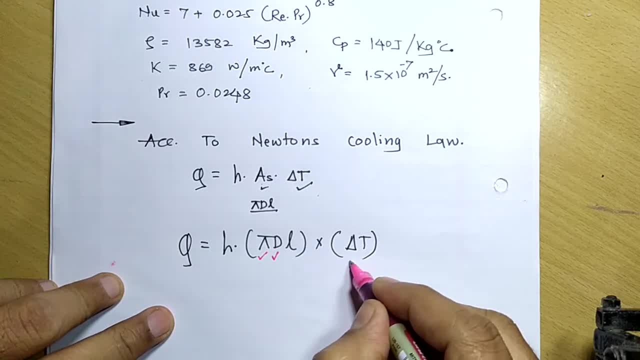 d is diameter given to you, that's 20 mm, and delta t is also knowing. just now we are seeing 50 minus 15 plus 35 by 2. i have to find out from this particular formula l, from this formula, what i have to find out. i have to find out here. so if i 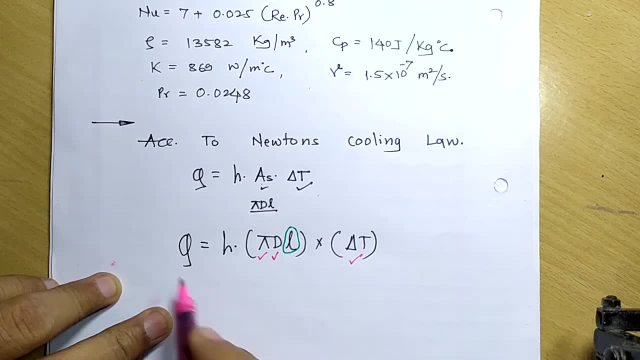 want value of l. if i want value of l, i should know all the terms in the this particular question. all the term means q, i should know h, i should know pi d delta t. out of that, pi d delta t is known, h is not known and q is also not known. so we have to determine one by one. we have to determine. 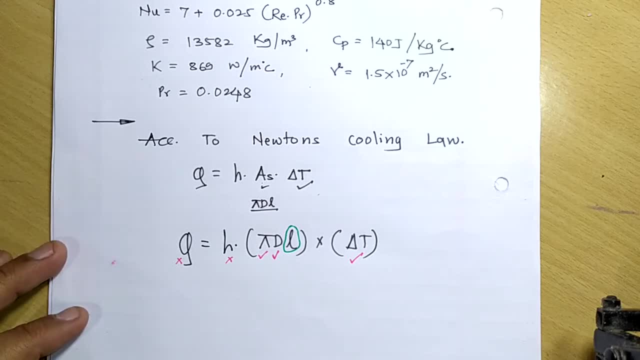 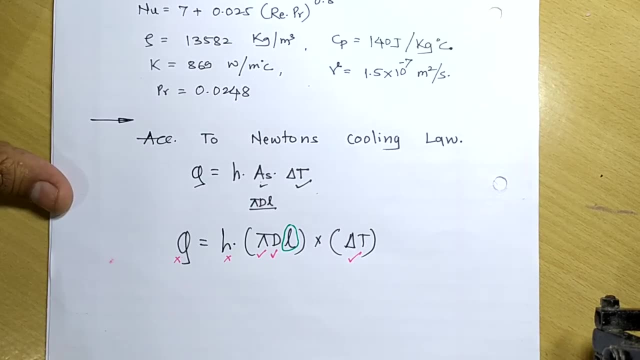 one by one, q and h. we have determined one by one, q and h. so what is q? now let's go determining for q and h. let's go q and h and that will give you a value of l. what is q? q is heat transferred from. 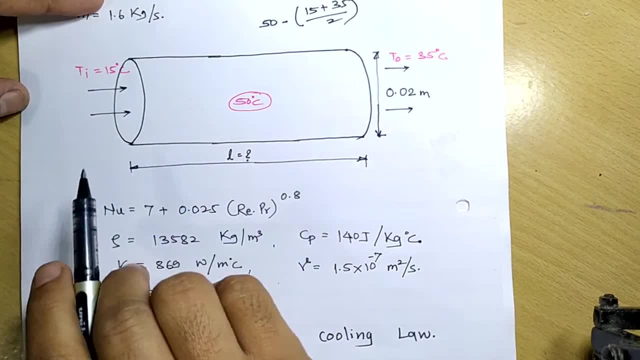 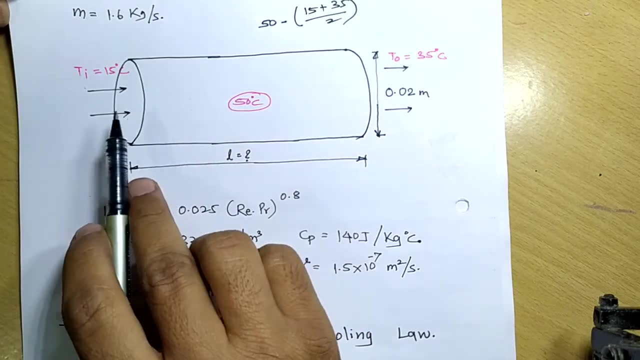 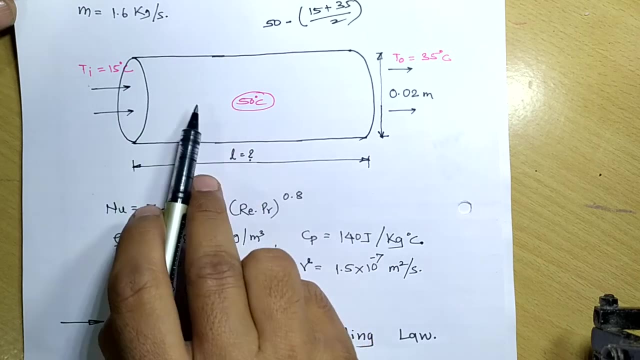 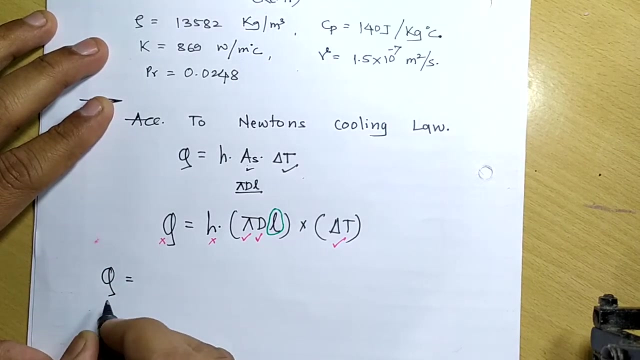 tube: heat transfer from tube to mercury. i can say that the q is heat transfer. heat rejected by tube is nothing but heat absorbed by the mercury. it's very clearly. i can say that heat rejected by tube is nothing but heat absorbed by the mercury. so i can write one sentence over here that heat transfer q is equal to heat rejected. 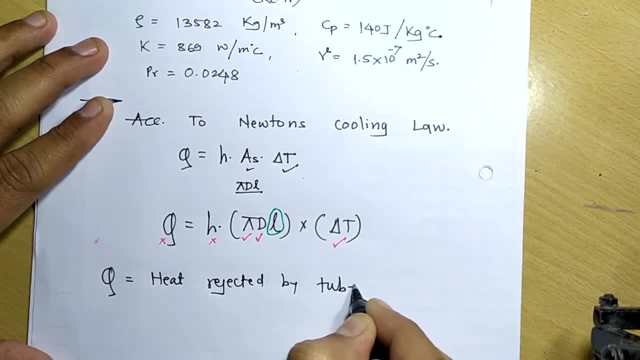 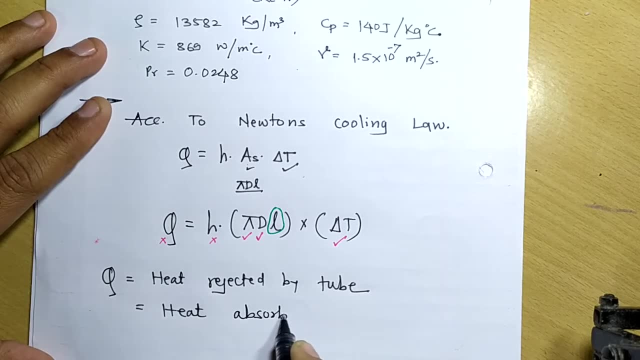 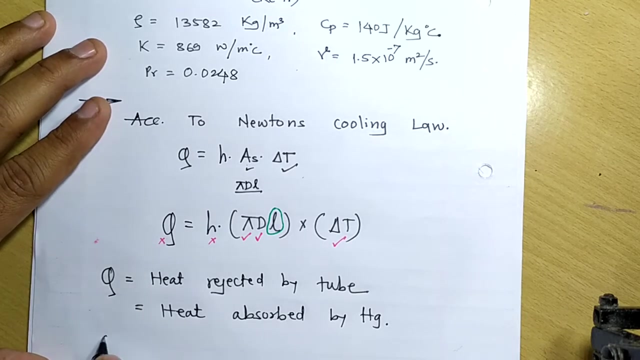 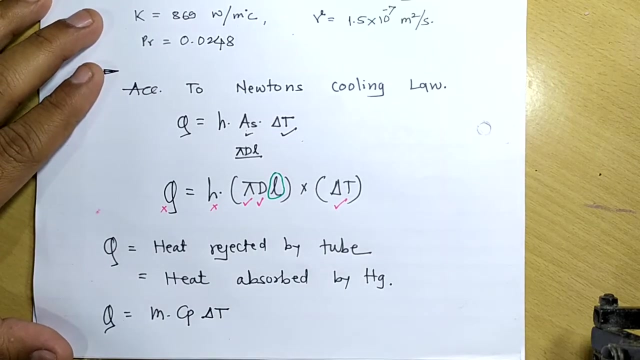 by tube r is equal to heat absorbed by mercury, that's h. now heat absorbed by hg. how we can write? heat absorbed by hg can be written as m, cp delta t. what is m cp delta t? that standard formula that can be taken from a thermodynamic m is mass. 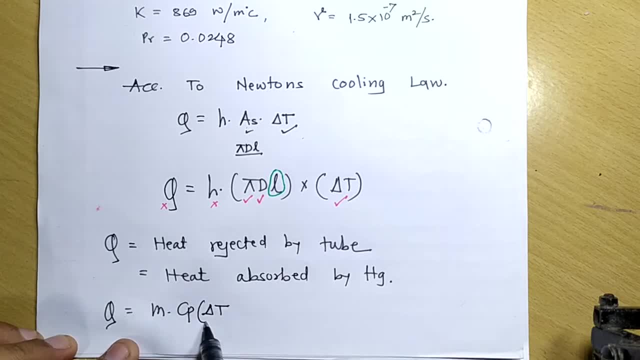 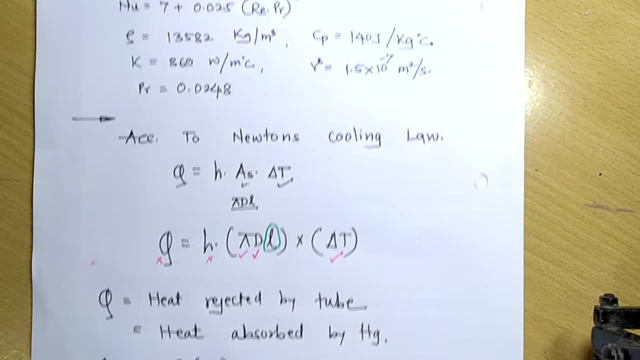 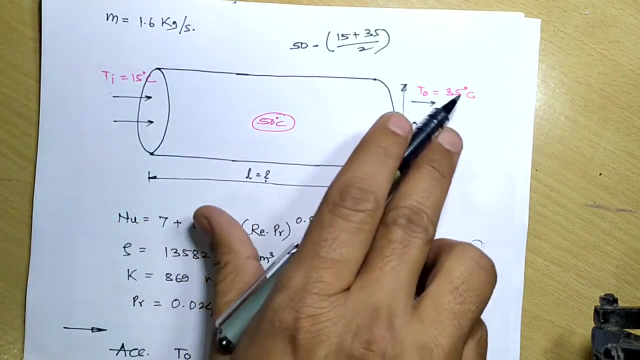 fluid. cp is a specific heat and delta t. this delta t is for hg, so for the mercury. what is the temperature difference that we are going to take it so for the hg? temperature is changing from 15 to 35, so delta t for hg will become 35 minus 15 and 35 minus 15 will become a 20. okay, so don't confuse here that. 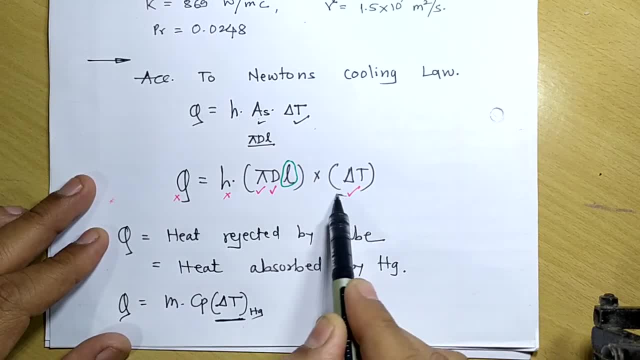 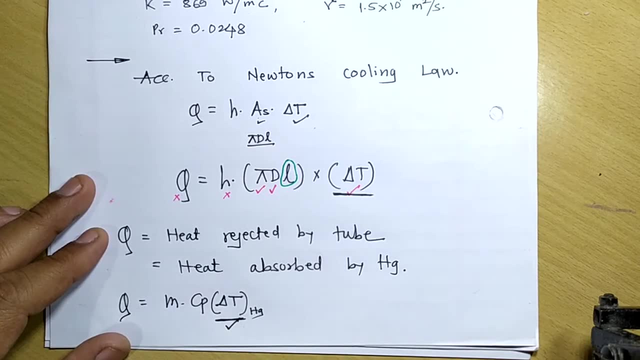 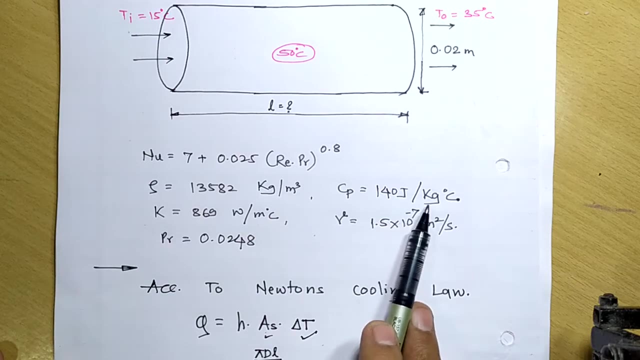 this delta t is only for hg, whereas this delta t is temperature difference between hot body and cold body. that's according to newton's cooling right. so i am knowing this. what is cp? cp is given in the problem. cp is equal to 140 joule per kg. per degree celsius mass polarity is given. so i am. 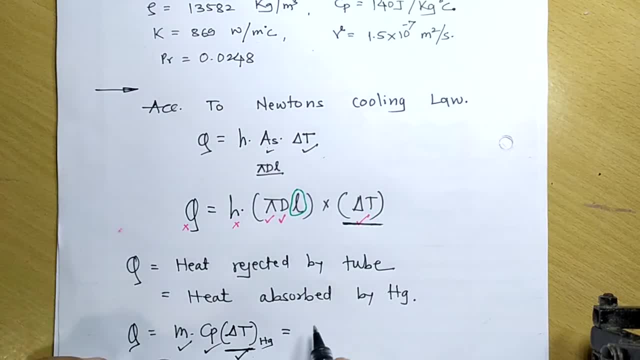 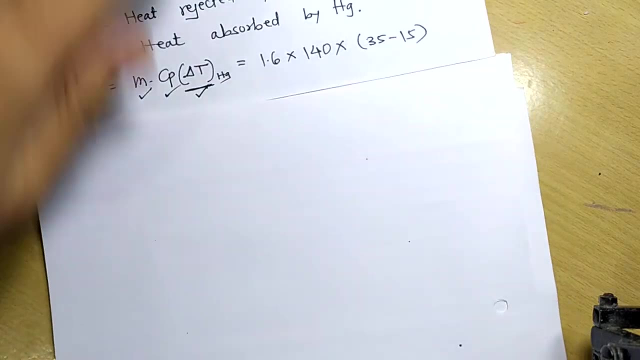 knowing all the terms, let's put the values and determine it. so mass polarity is 1.6, cp given to you is 140 and delta t is a 35 minus 15. so with this you can do the calculation and after doing calculation you can write what is. 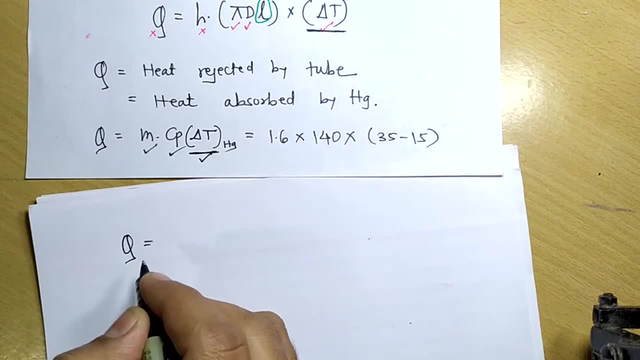 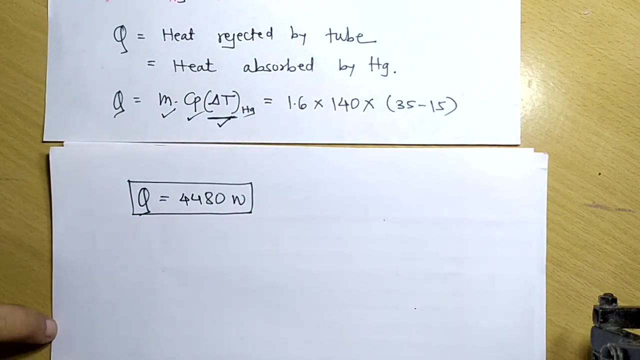 the value of q. okay, so let me write value of q. the q will come to be 4480 watt. that's the value of q. so we have got first answer. that is the q. we have got first answer. that is the q. now going to the second answer: what? 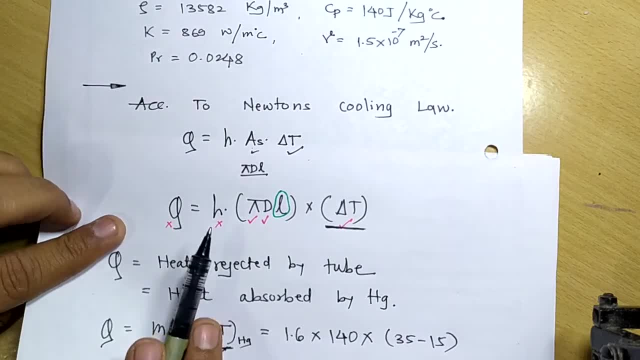 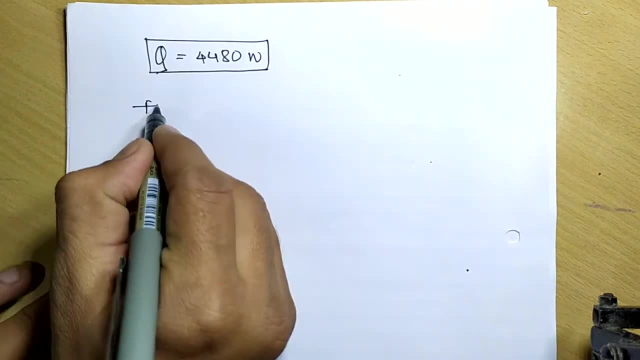 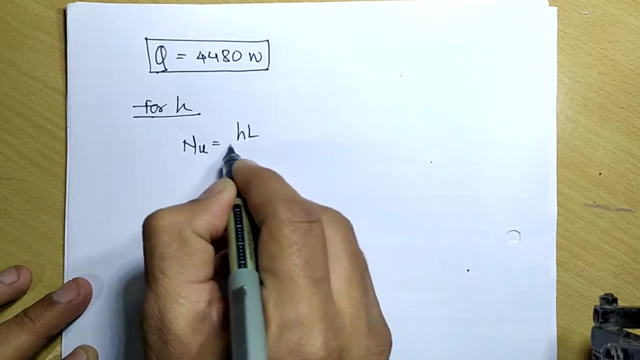 i have to determine. i have to determine this h, i have to determine h. so how we can determine h, let's see how we can determine h that we are going to see. so for h, for h, i can use a formula that nusselt number is equal to h, l by k. what is l, l is characteristic h, l, c by k. from this, 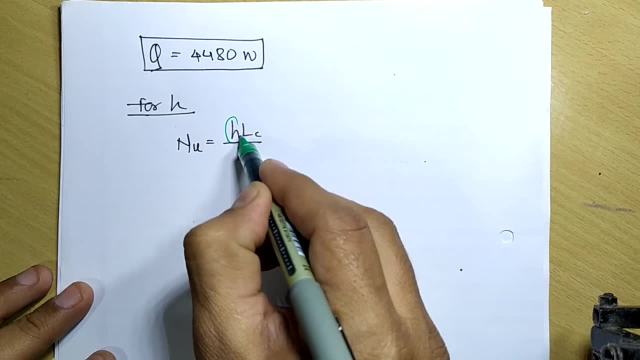 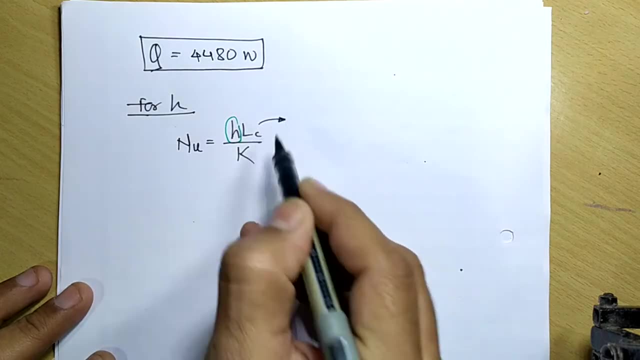 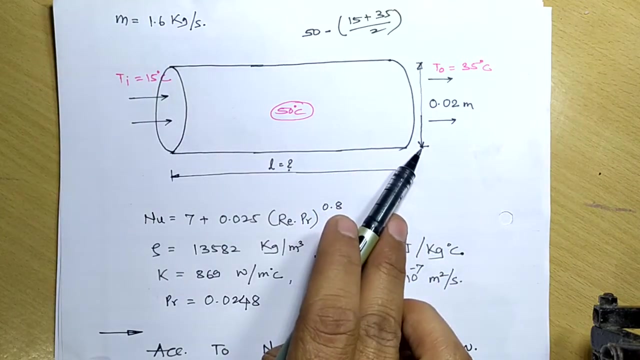 i can determine h if i am knowing all other term. what is all other term? that is l, c, k and nusselt number. what is l, c, l, c is a characteristic length. in this case, what is characteristic length when we are having a tube and internal flow is there? the diameter is a characteristic length. so 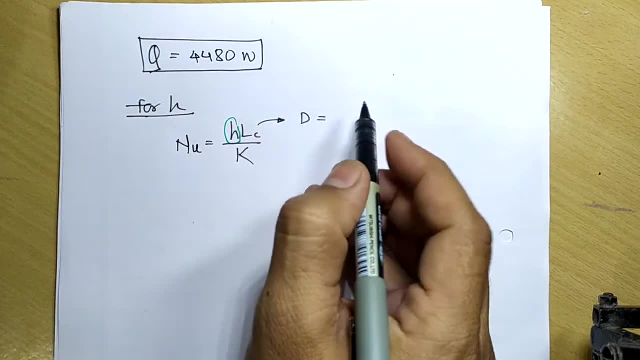 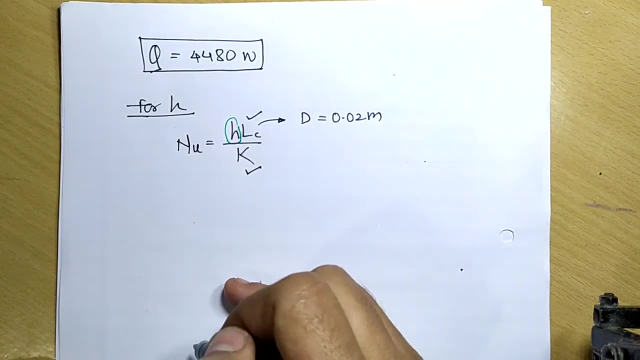 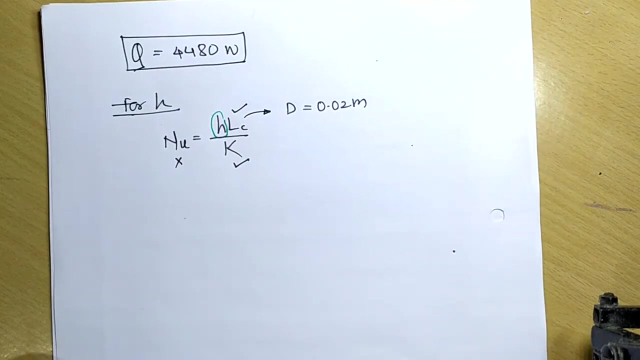 here l c is nothing but diameter, which is nothing but given in the problem as a point zero two meter. so i am knowing l c. i am knowing k is given in the problem which is eight six nine watt per meter per degree, but i don't know nusselt number. i don't know nusselt. 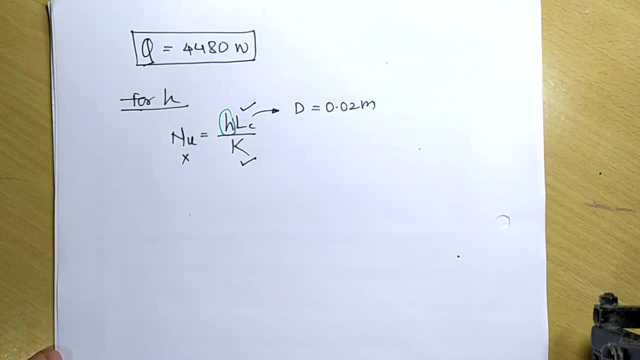 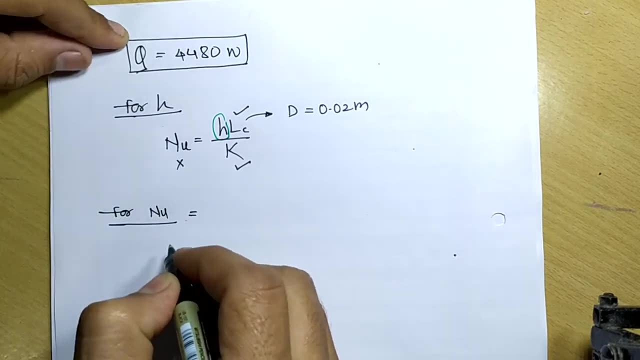 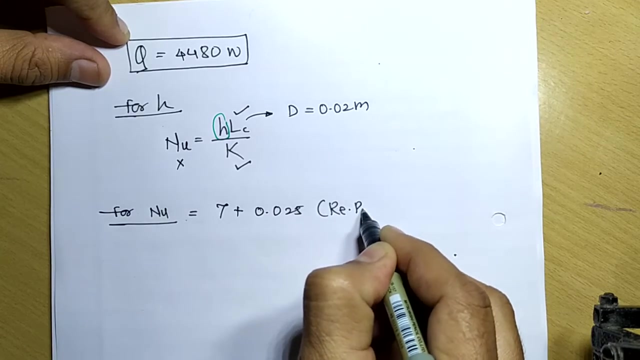 number. so how to determine nusselt number? that we have to check it, that we have to check it. so for nusselt number, for nusselt number, what i am going to do. they have given one relation that 7 plus 0.025 re into pr raised to 0.8. by using this i can determine what nusselt number. 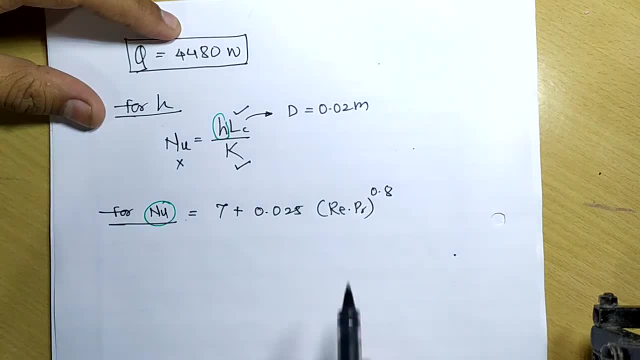 i can determine nusselt number, but for that i must know re and pr. out of that, pr is directly given in the problem, which is 0.0248. now, what about re, re, i don't know. so for renal number. for renal number, i can use a simple. 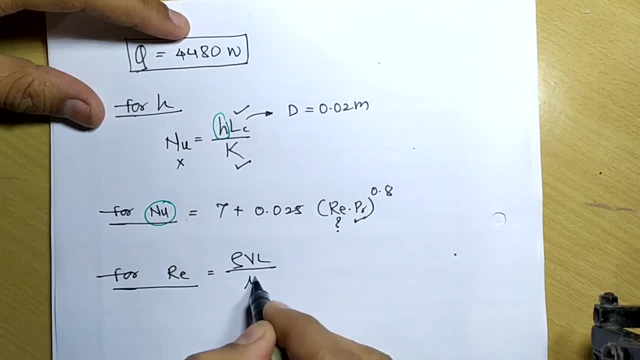 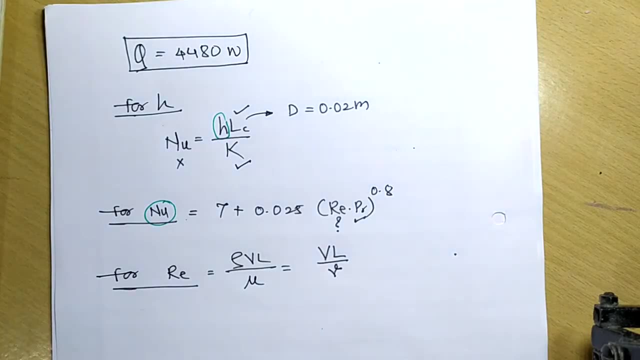 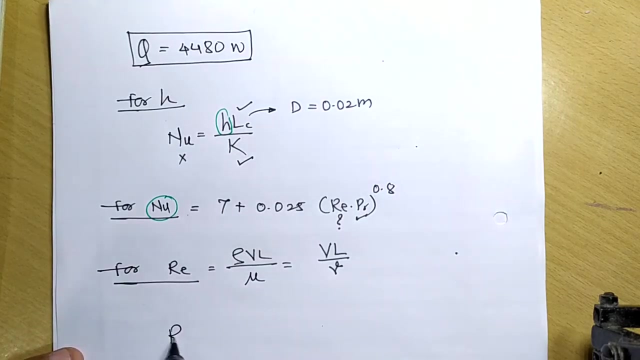 formula rho, v? l by mu or v? l by nu, so i can use any one formula: v? l by nu, right? so i can determine the renal number, re, and i can put over here, i can put over. i can determine nusselt number. i can put nusselt number here and i can determine the h. so let's follow that particular. 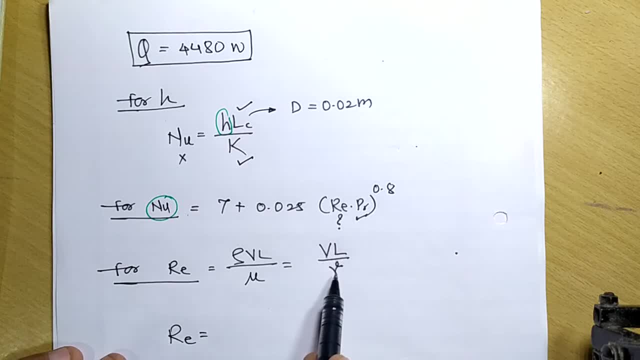 process. so re is v? l upon nu. what is v? v is the velocity, v is what velocity of fluid flowing through the pipeline. okay, so let's determine first of all v, because i don't know. okay, lc characteristic length is known, nu is not. i don't know v. so 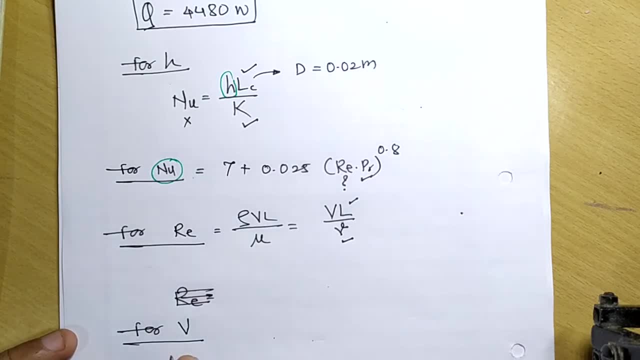 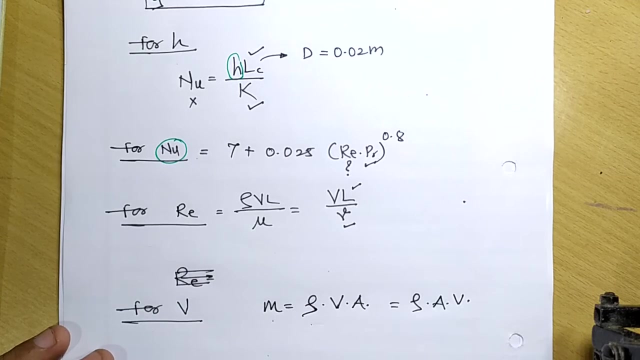 for v. i am going to use one standard equation, and that standard equation is: what? mass flow rate is equal to rho v, a or some of the book. we write a rho a- v. the meaning is same. so mass flow rate is equal to rho a- v. rho is density, a is a cross-sectional area and v is the velocity. 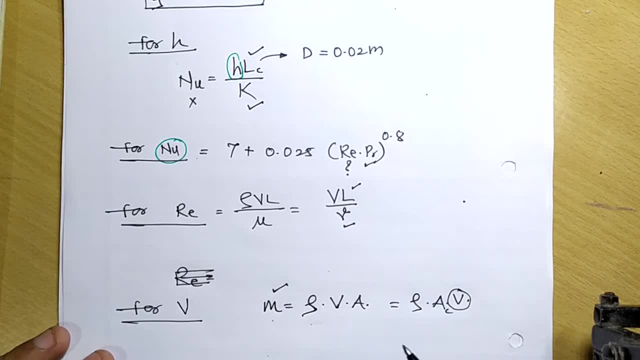 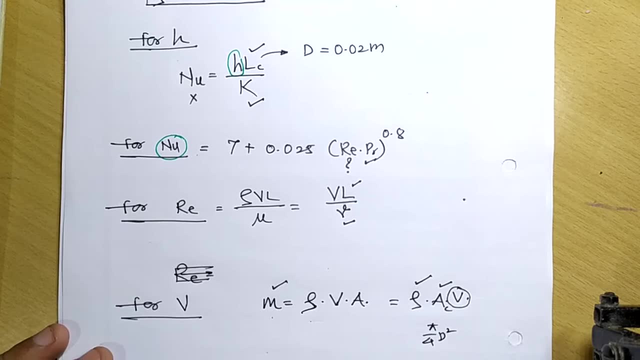 from this i can determine a velocity, because i know mass flow rate, i know density, i know cross-sectional area is pi by 4 d square, pi by 4 d square, that i can keep. i can determine velocity. this velocity i can keep here. determine renal number: this renal number i can keep here. determine nusselt number. 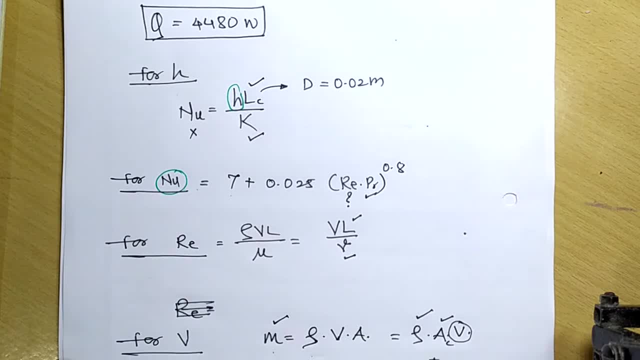 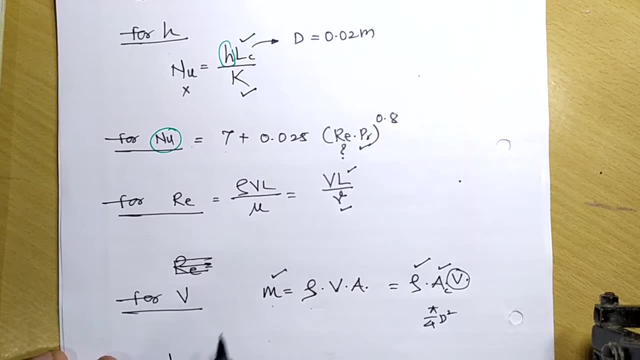 this nusselt number i can keep here, i can determine h and then i can go for the actual solution. now task is determine velocity first. to determine velocity, let's put all the values: mass is 1.6, density given. let me check how much density is given. density given to u. 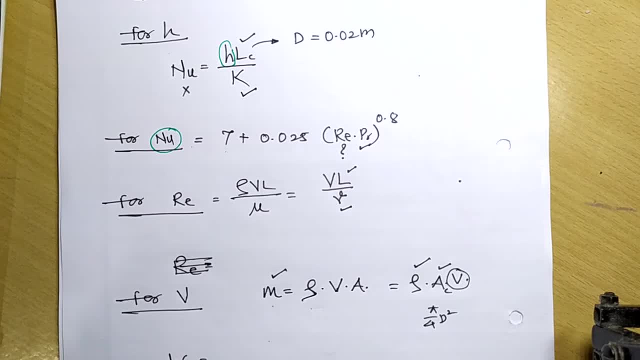 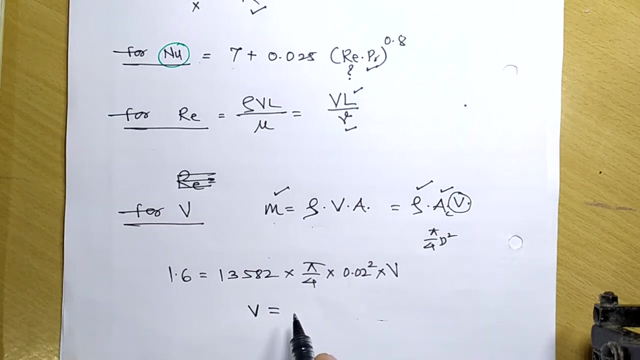 1, 3, 5, 8, 2 into cross-sectional area is pi by 4 d square d is 0.02 square into v. from this i can determine velocity v and that velocity should come to be 0.3749 meter per second. and that's what we have got. velocity. now, this velocity i have to. 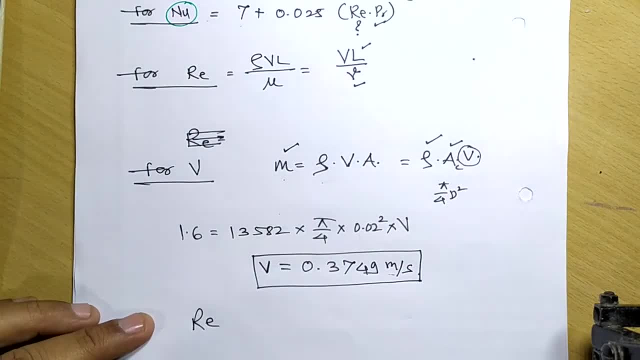 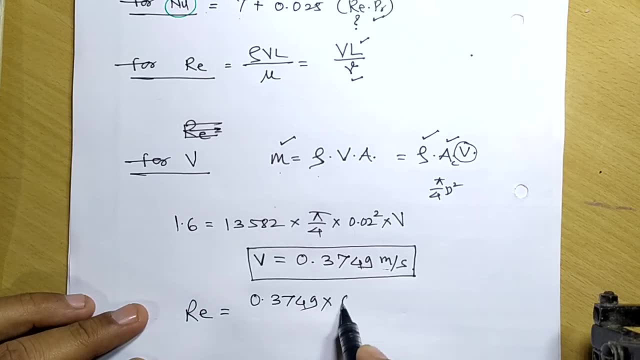 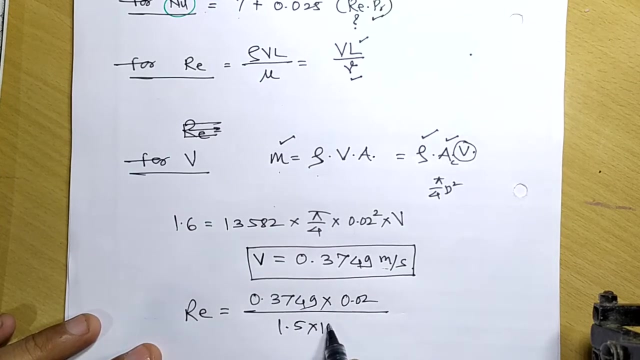 keep here and determine renal number. so renal number re. renal number re is equal to v. that is 0.3749 into l is 0.02 divided by nu nu is given to you how much is nu? nu is 1.5 into 10 raised to. 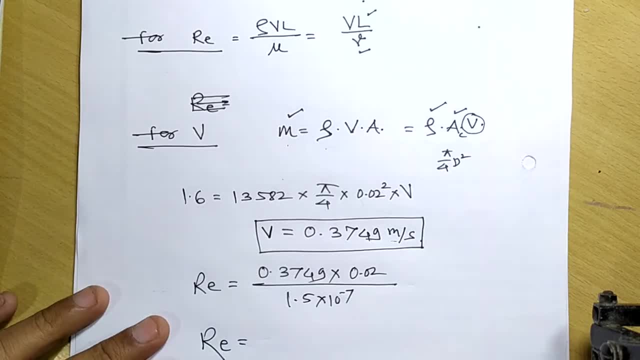 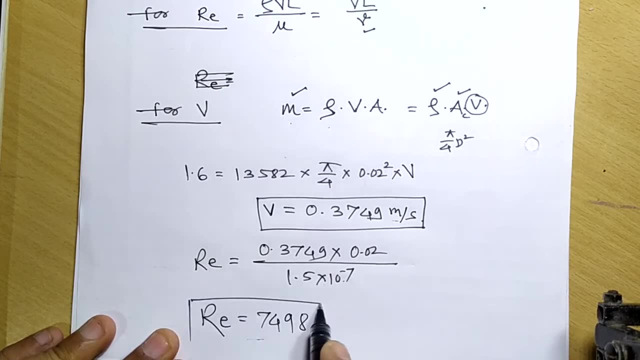 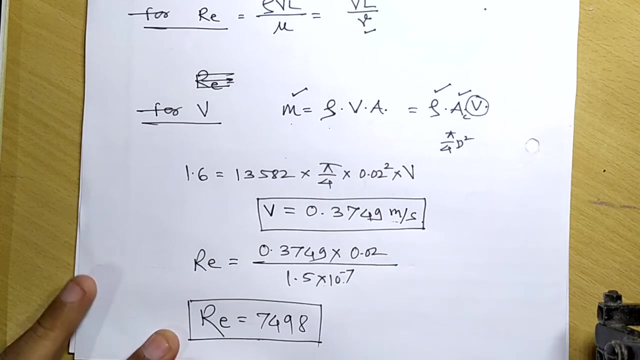 minus 7.. renal number can be determined. so the re will come 7498. so that renal number we have determined. now we have determined the renal number. now let's go for determining nusselt number, because now we have determined renal number put up here and determine the nusselt number. so i am going to put all values. 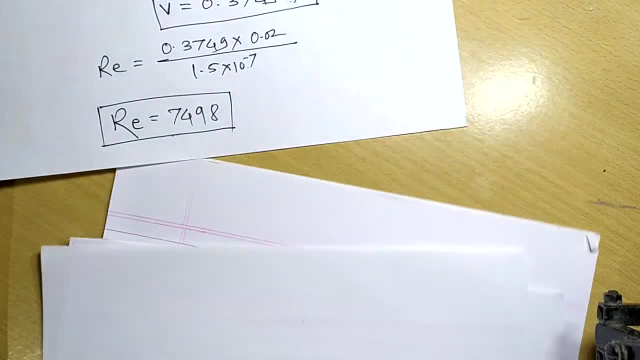 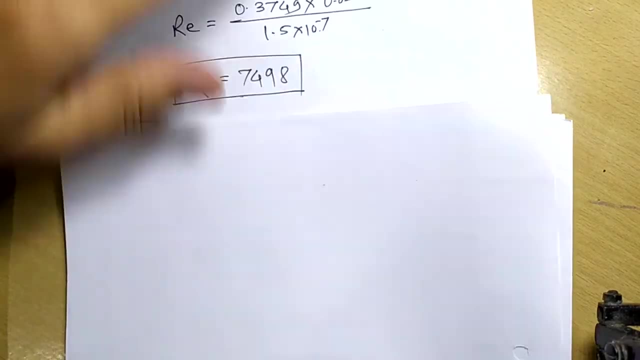 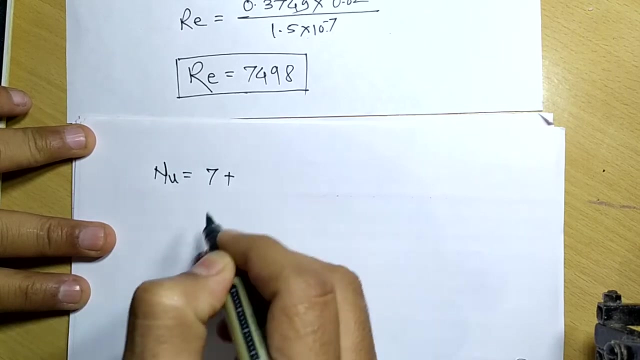 over here: renal number and parental number. so let's put it. let's put it, so the value will come. the value will come as like this: let me write over here as like this: that nusselt number is equal to. nusselt number is equal to 7 pulse plus. 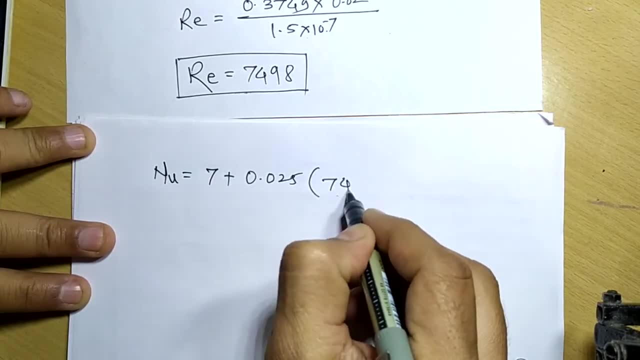 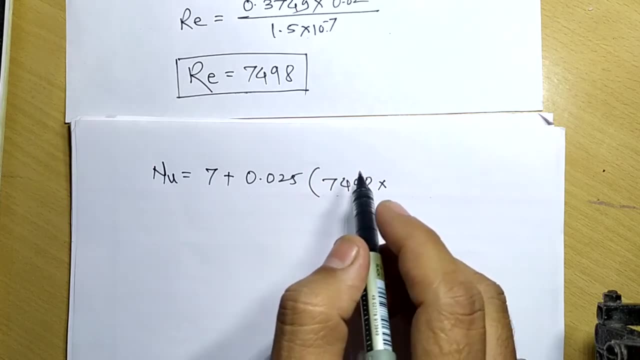 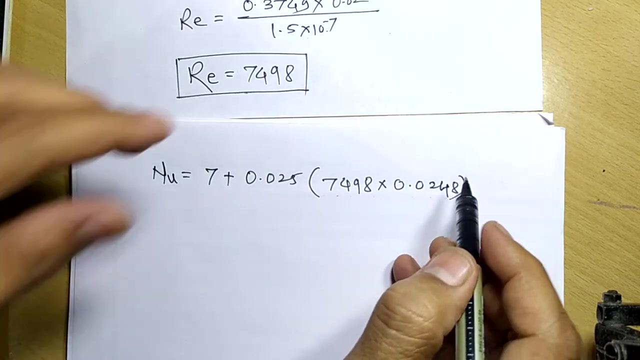 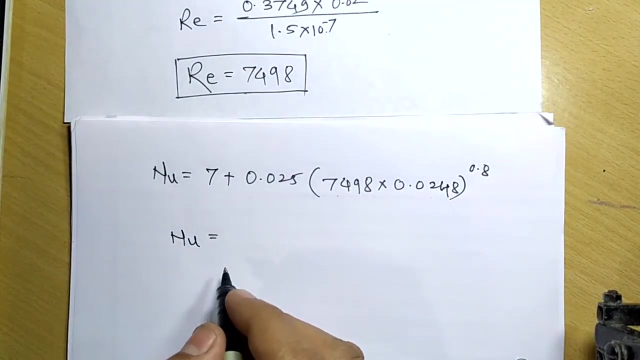 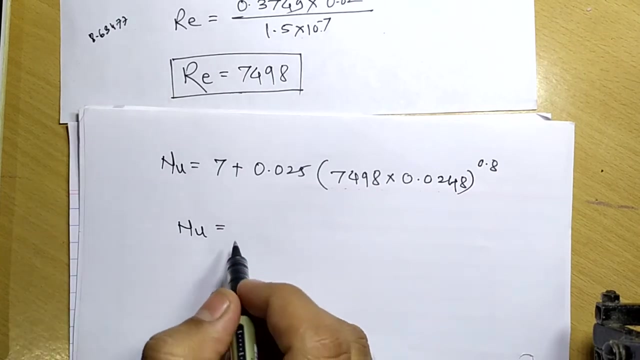 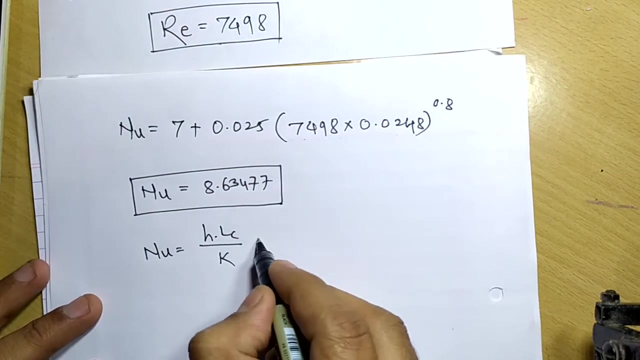 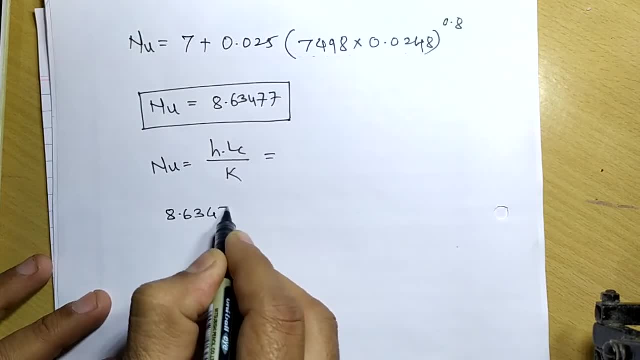 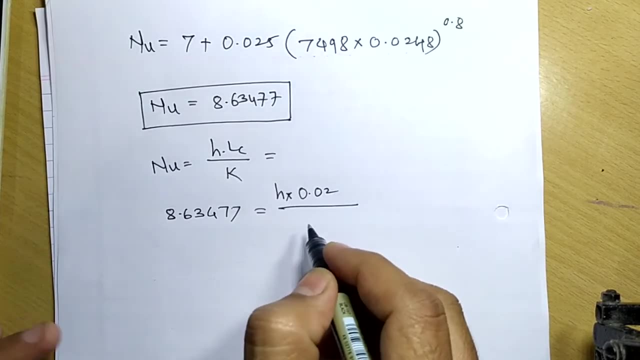 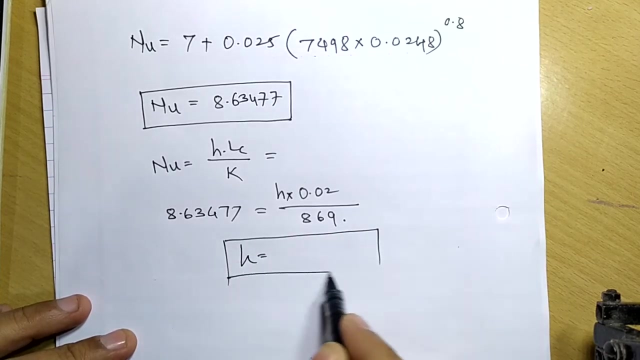